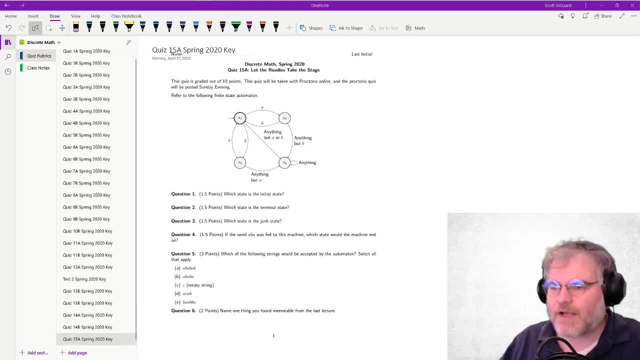 Thank you for watching, Anyway. so I don't know why this thing is doing that. Okay, well, now it's doing the thing where it, you know, doesn't want to. it thinks black is a color, is chroma, key green, and I don't know how to fix it. 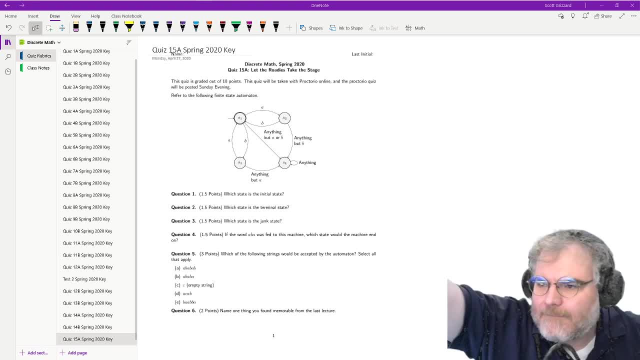 Let's see if I open the window. Hey, that helps A little bit. Okay, so technical issues. sorry about that, Anyway. So today we're going to be talking about non-deterministic FSAs, finite state automata. 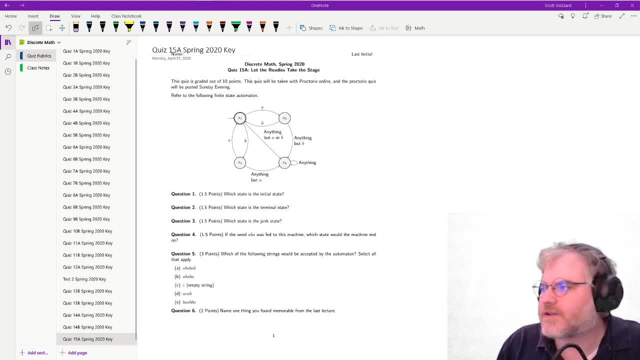 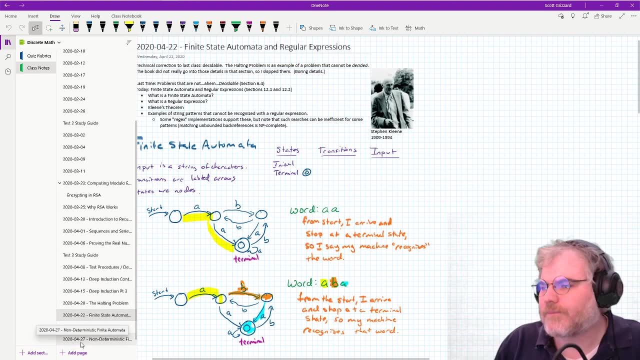 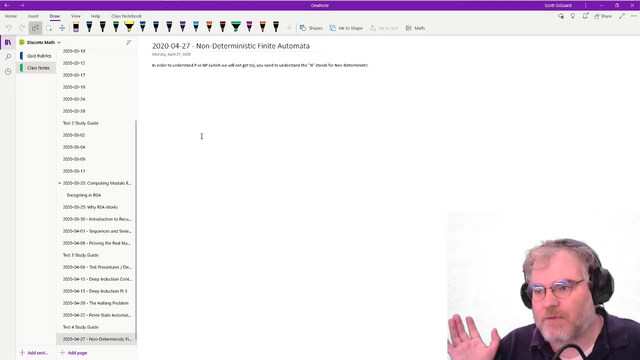 Now the issue is that I should switch to the class notes for that. So last time we talked about finite state automata and we're going to go over the quiz, But today we're going to talk about, in order to understand P versus NP, which we won't get to probably. I might get to it shortly. 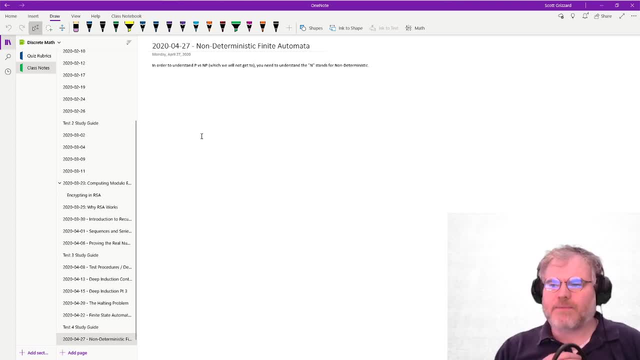 I might get to it at the very end a little bit, But I'm not going to be able to do P versus NP the whole thing. So in order to talk about P versus NP, you have to understand what a non-deterministic Turing machine is. 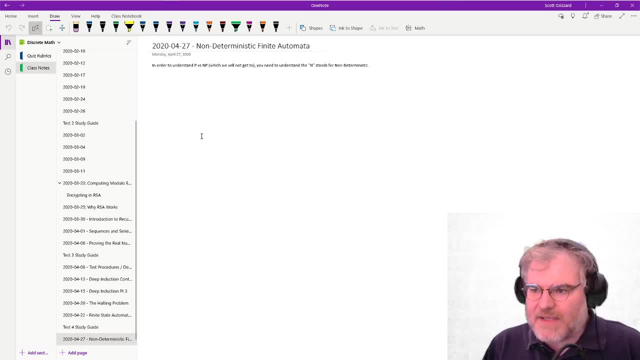 Which means you have to understand what a non-deterministic thing is, Because that's what the N in NP means: non-deterministic. So that's what we're going to do. That's actually the confusing part of the problem. 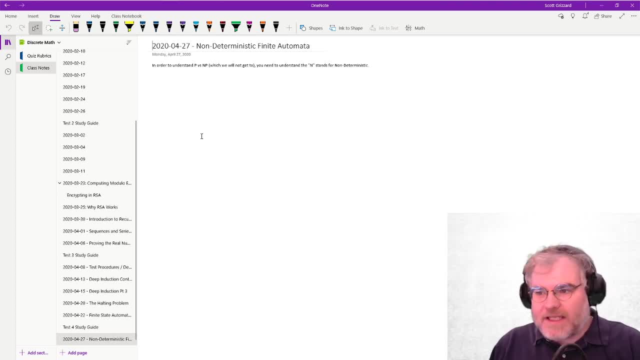 I mean problem's unsolved right. So if you want a million dollars, figure out if P and NP are the same thing, Okay, But there's a million, There's a million dollar bounty on that one. But if you can provide a proof one way or the other, 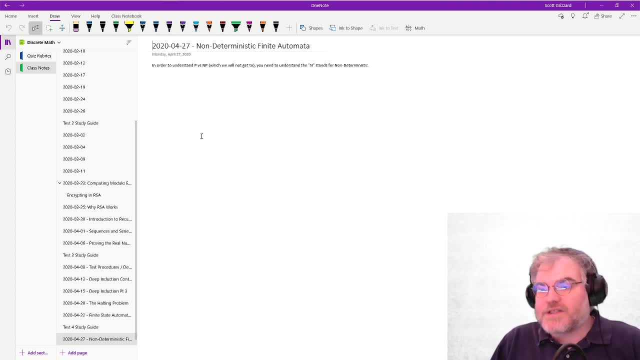 We just don't know. And worse, according to Godel's theorem, it may not even be, you know, decidable. So you know there may not be an answer, But if you could prove that you'd also get the money. 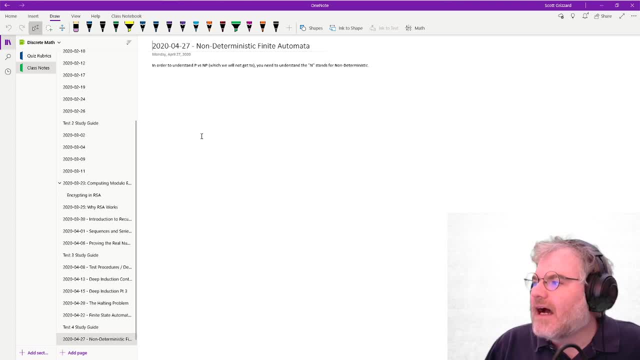 Anyway. so that's what we're going to be talking about today, Which is this thing that you have to understand, which is the non-deterministic part. But we don't have like three more classes. This is our last class. 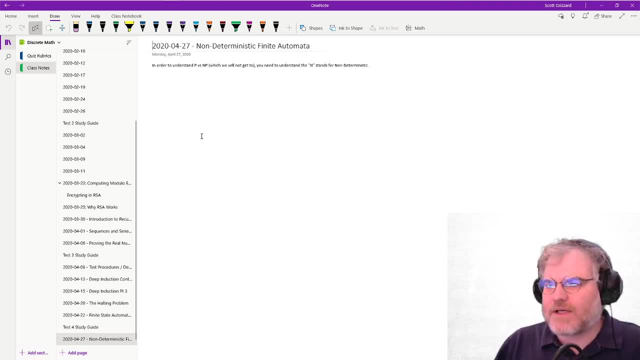 Sad, This is our last class, So I'm just going to get to non-deterministic finite automata And then the. if you're interested in P versus NP and you may see it in your class, you'll have a leg up knowing, because now you understand what a non-deterministic machine is. 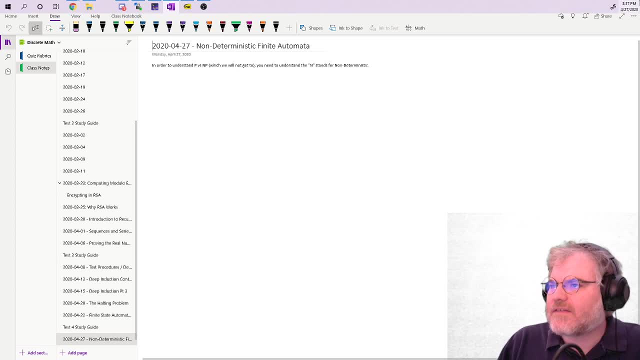 So that's the plan. Are there any questions in chat? Do do, do, do. Okay, So, yeah, Sorry, I was three minutes late, So this is today, Yes, And the TA is telling us all about the millennial problems and the prizes and the fact that one of them got turned down. 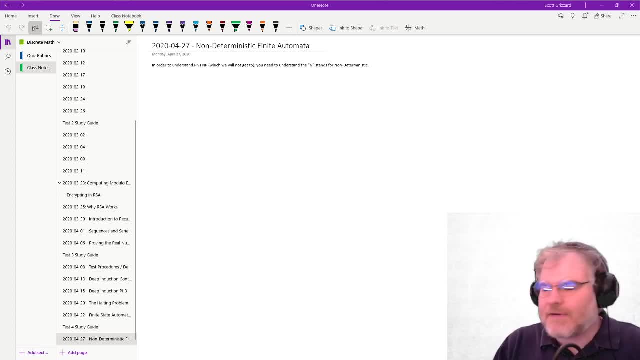 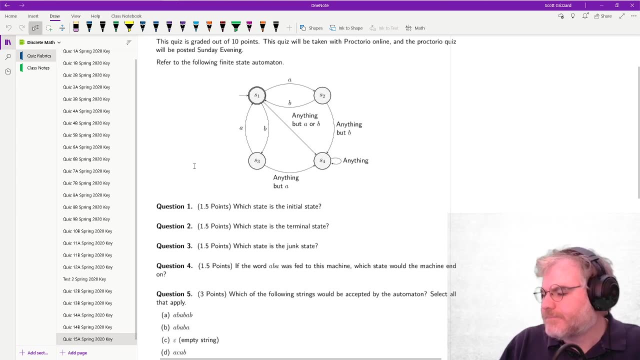 So, okay, Very cool. Anyway, let's talk about the quiz. So our last little quiz It's about finance State automata And people have been telling me they're kind of fun. I think they're kind of fun too. 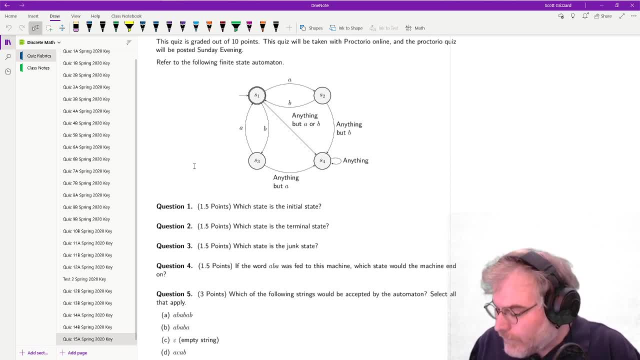 This is why I wanted to do them, Because they're useful- heaven forbid- and they're kind of fun. That's the calculus notebook, Okay, So what state is the initial state? This is actually it should be. which states are initial states, because a machine can have or no. I'm sorry this, this is correct. 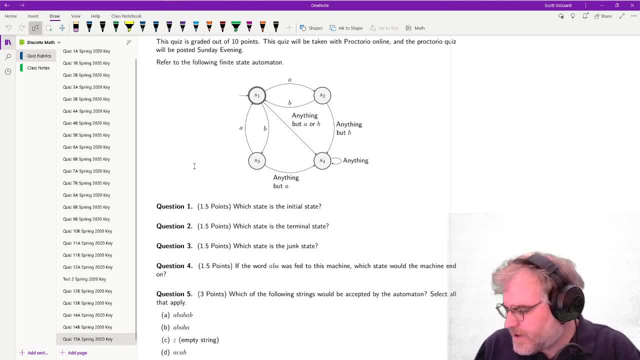 Which state is the initial state? There's only one for a deterministic machine and that's S1.. How do I know that It's got this little arrow there? It may have start. Some of them have start here written there. This one didn't. 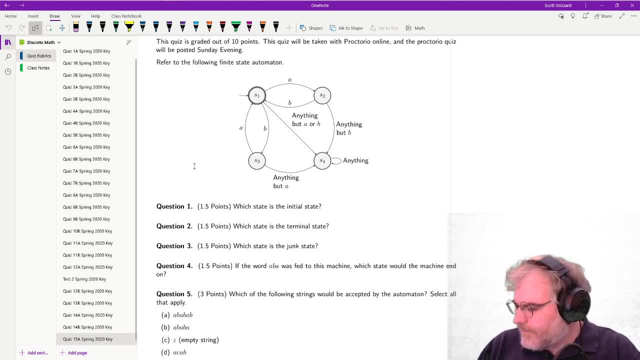 It's just got the little arrow there, So that's not I know where I begin. How do we feel about that? So let's do that one to five. Okay Now, which state is the terminal state? Now, it's important to note that even a deterministic finite state, automata can have more than one terminal state. 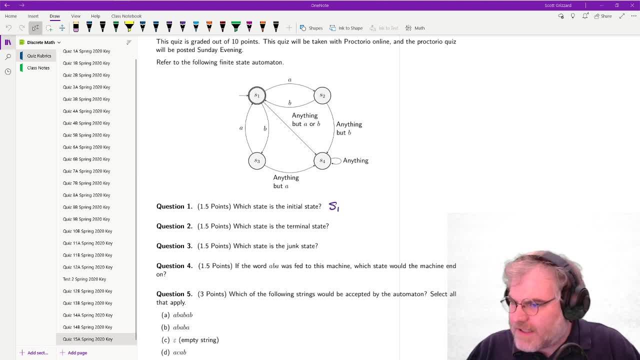 Okay, But here the terminal state was is indicated by that second circle, and it's that It's also known as the accepting state. all of those things, All right. So how do we feel about that, The, the terminal state or the accepting state being being designated by that that double, that double circle on it? 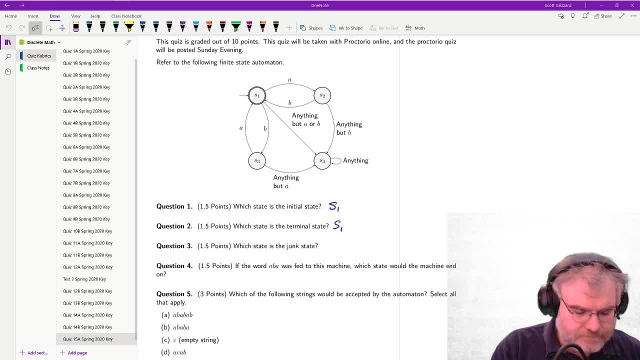 It's an order of decorum and this is, this is a, it's a plus. You know, this is, this is it's a. Okay, Now, if I'm going to do this with a, a prism, So let's say that this thing is my. my I'm gonna do the truth. check here. 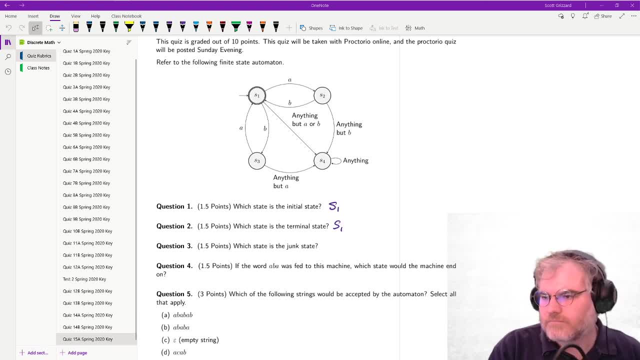 So let's have it check. Here we go. Well, what about this? It's the state. Well, what about it? The state is my, my, this is the state. Okay, Now, which state is the junk state? 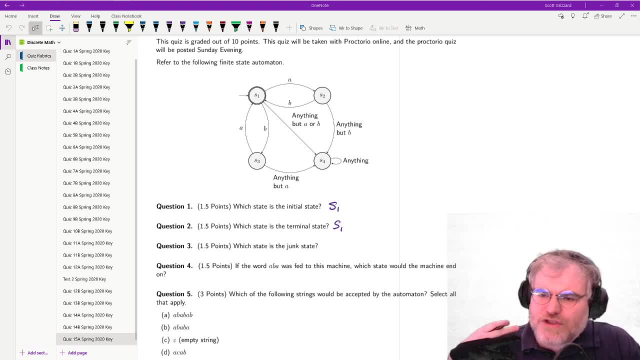 It's the state. Now let's look for one. So you're talking about, like the state of the, the, the, the, the PPS. Well, the junk state is the place where everything lands right. 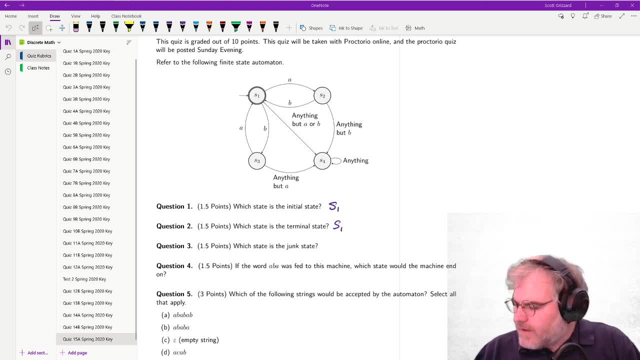 It's Hotel California right here. all right, there's, it's all it's only got. uh, you know it's got all of these ways to get in and then you just loop inside, right, so we'll call that one hotel california. you can check out anytime you like, but you can never leave. 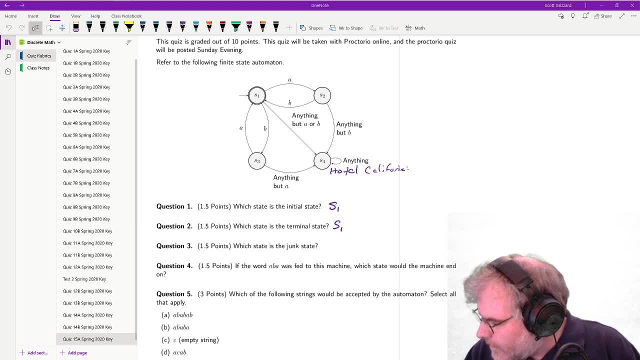 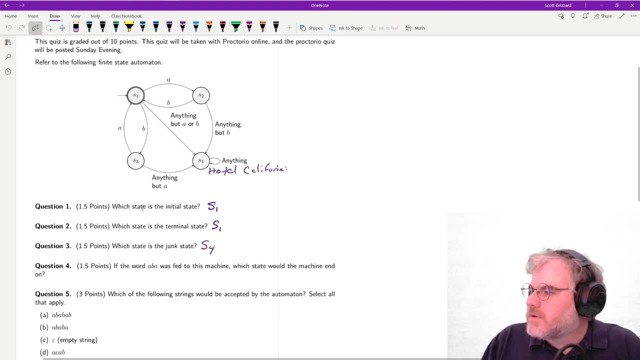 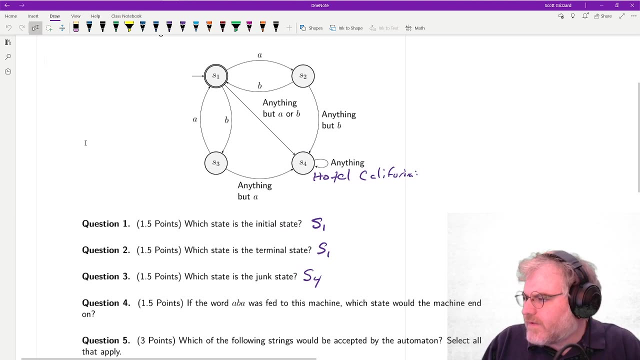 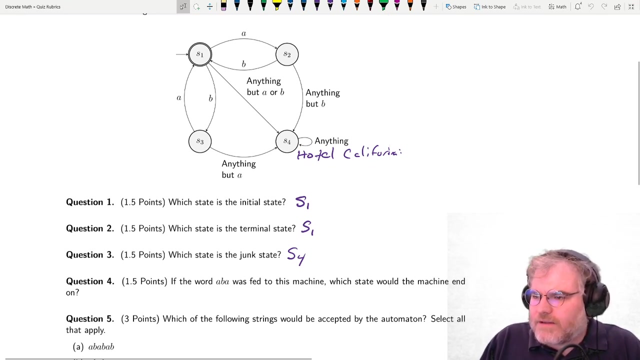 uh-huh, so that's s4. how do we feel about that? one to five. i know the book didn't go into junk states very well and i kind of like breezed it a little bit, but how do we feel about that? you, you, okay. the idea of the junk state here is that it accepts everything. 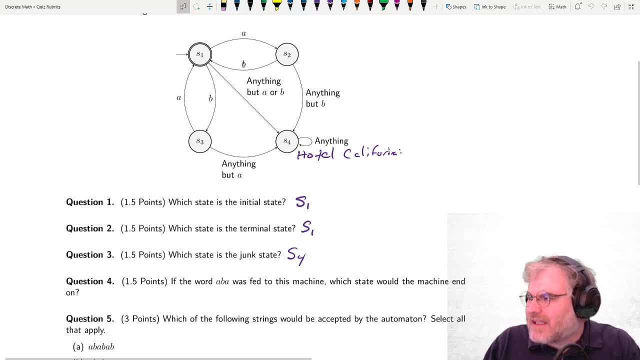 um, that doesn't have a valid entry right. so here, if i had a, a, i'd go a here, but then i wouldn't go b, i'd go to anywhere else and that lands into this junk state here. but it's not that just accepts, it's that it loops itself for everything. so anytime i get i can't leave the state. it's not. 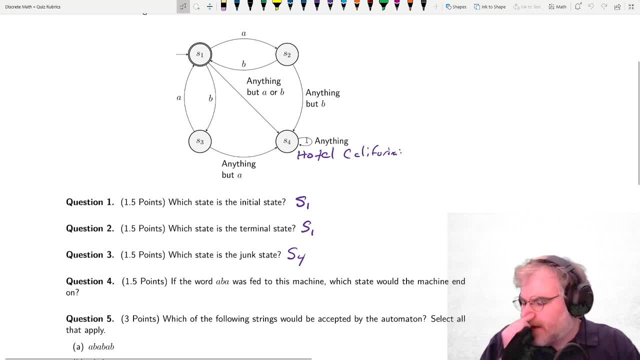 a terminal state. it's just a state that accepts everything, just where the junk winds up. okay, it's a trap, all right now. if i feed aba into this machine, where do i wind up? well, here's a, b, a. i wind up at s2. how do we feel about that? one to five. 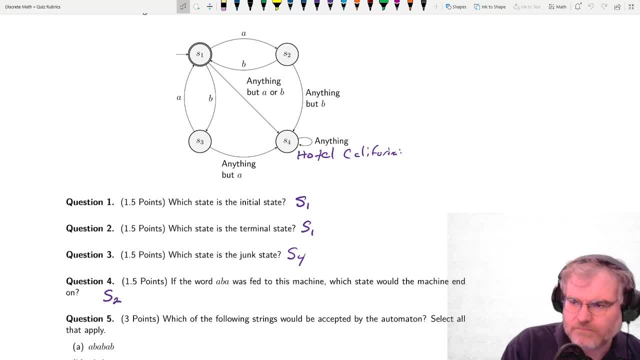 okay, there's a question in chat: is it the equivalent of an error message in a program? it can be, but it's just, it's a. it's the equivalent of a: not match will never match thing. um, i mean, it's not just an error message, it's. you know, it's not just an error message, it's. 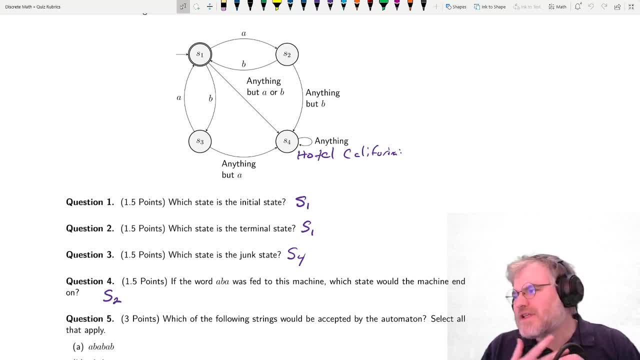 something like you know i could distinguish, i could. i could say that the machine is only supposed to want take a's and b's and then have like an error message state where you know if you throw anything but an a or b and it goes no um and whether or not you call an error valid a valid. 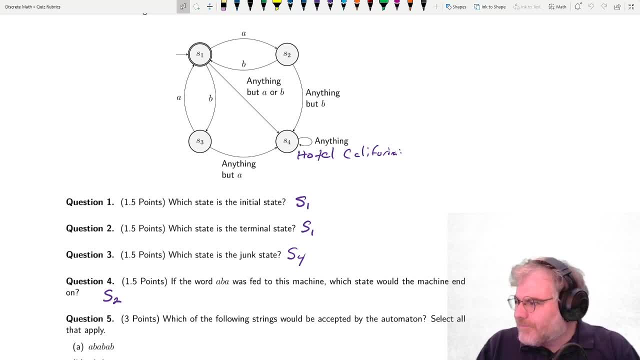 accept, is you know? another question? um, i wouldn't. it's called an arrow, but the idea is that it's the thing where, if you're not going to match, you just wind up there and then i'm not going to spend any more computing resources dealing with it. i'm. 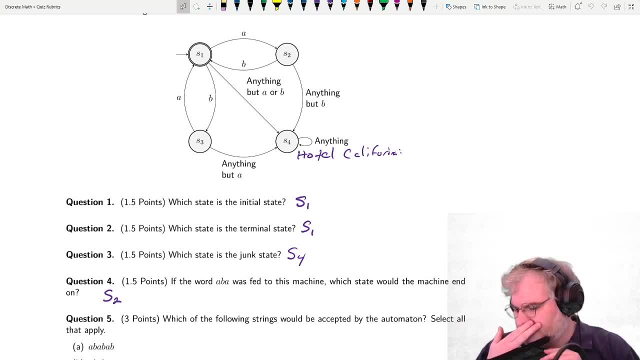 done with it. okay now: a, b, a, b a, b. so if i go a, b, a, b a, b, i wind up at a terminal state- s1, so that's a yes. but the next one, a, b, a, b, a, goes a, b, a, b a and i wind up at s2 and that's a no. 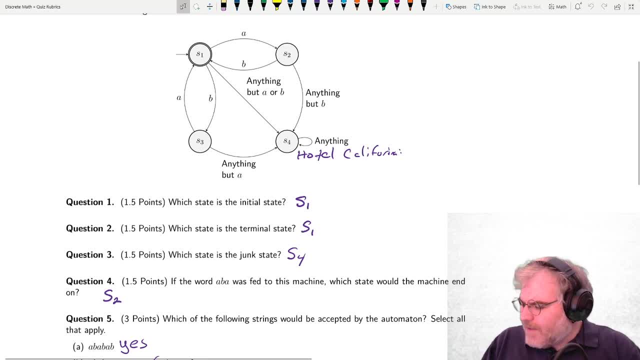 because s2 is not accepting. so how do we feel about the first part of question? five there, one to five, yeah. so the question in chat is, when it says accepted, that means a terminal state, yes, or an accepting state? i don't remember which one. does your book use the the literature, so i've got uh. 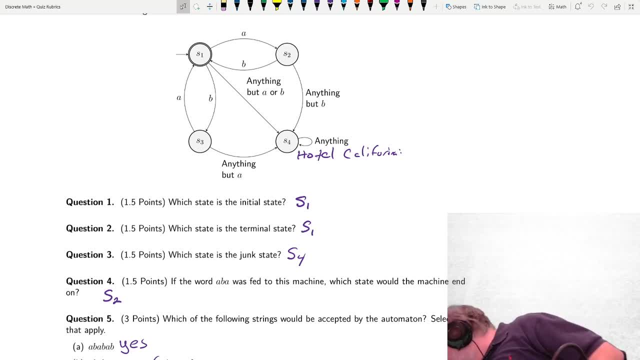 when we started getting into this, i dug out the old uh, the old uh, pop crop phenomenon. um, which has different terminology than the book does. oh sorry, i just hit the microphone again. this microphone picks up everything, i swear: regular expression, finite state, automaton, accepting. so your book uses the word accepting, uh, the other book uses the word terminal. same thing. 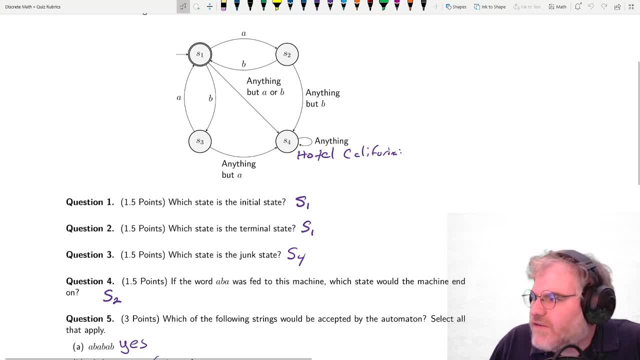 all right, the empty string. this one's tricky. i start here and then where do i go? well, nowhere, right. i started s1, that's the initial state, and then i go nowhere. i end at s1. that means i accept. right, that's an accepting or a terminal state. 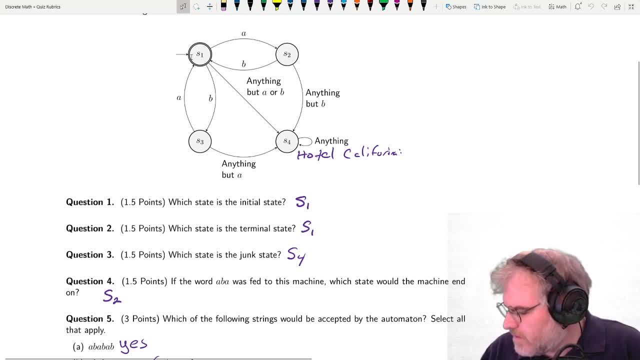 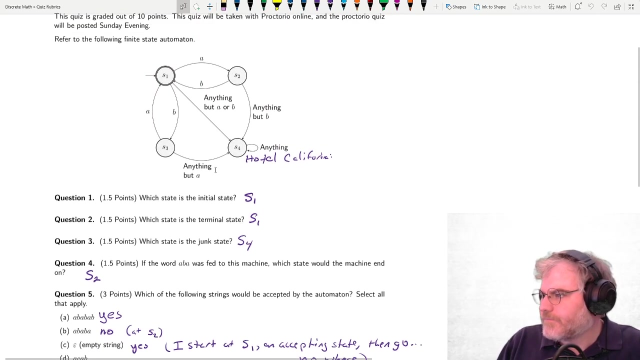 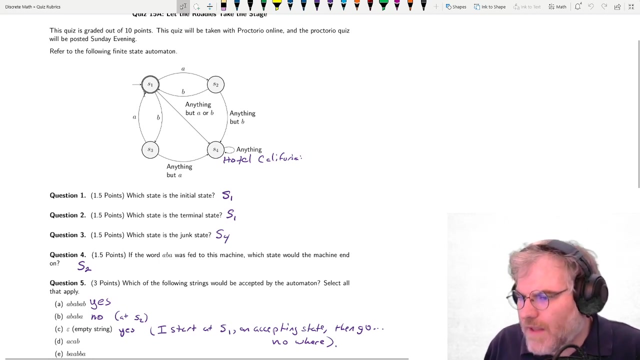 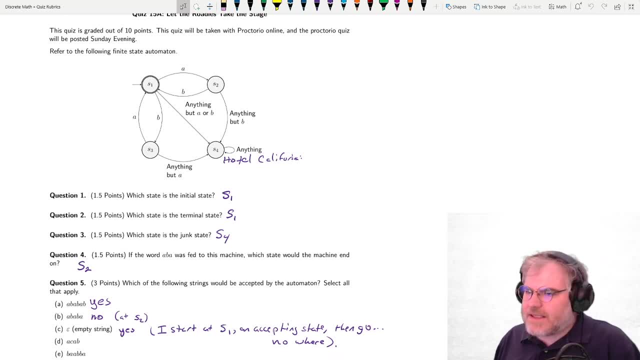 how do we feel about that one to five, this idea that the empty string starts at starts and goes nowhere, there's nothing to process. there's nothing to process. process for, for, for, for Now, if my finite automata had its accepting state, did not have S1 as an accepting state. 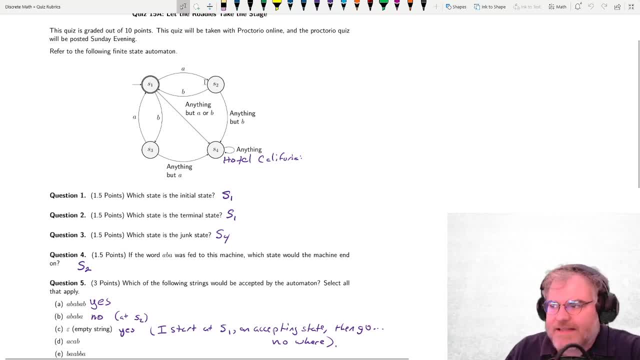 but had S2 as an accepting state, it would not accept, correct, Because it didn't go anywhere. Okay, Now the next one: A C A, B A C. I'm in the junk state, Okay, and the next one: B A, A, B, B A, B A, A, B, B A. yes, 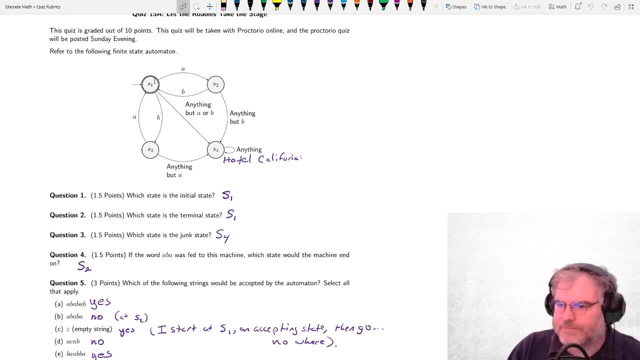 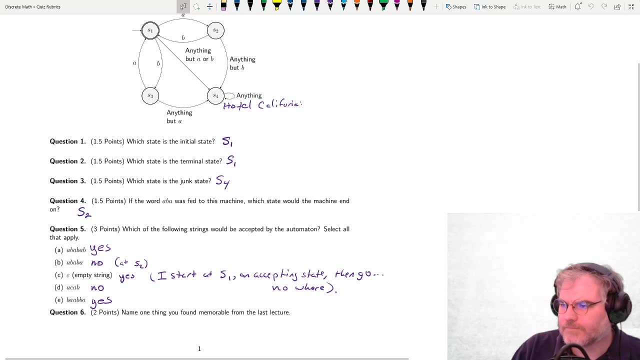 How do we feel about those last two? one to five, Okay, Okay. Okay, A C A B is like this: It goes: A, C A B, Okay, Any other questions? Any other questions? Well, the second A follows this: anything path. right. 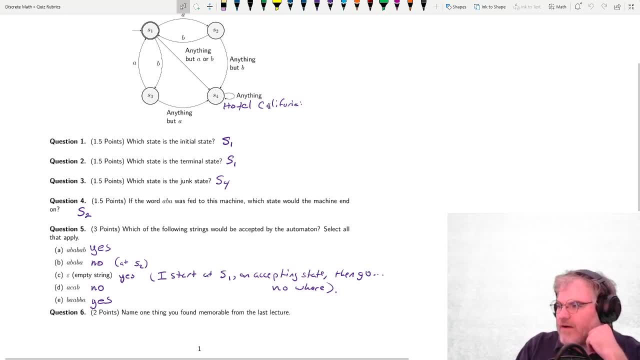 Because A is something. So the second A goes anything, anything, anything. You know, once I wind up in this state, anything comes back. So the question was: was the second A goes nowhere? Well, it does. It goes along the anything path because A is a thing and it just goes back to junk. 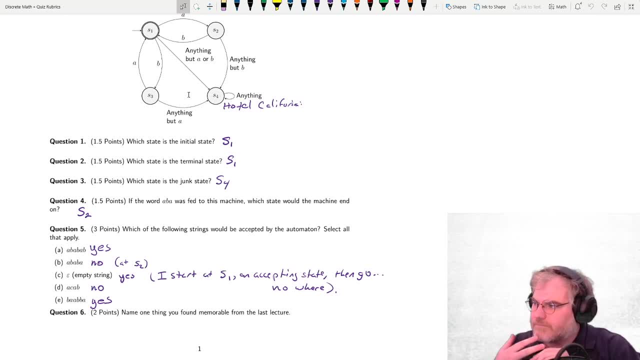 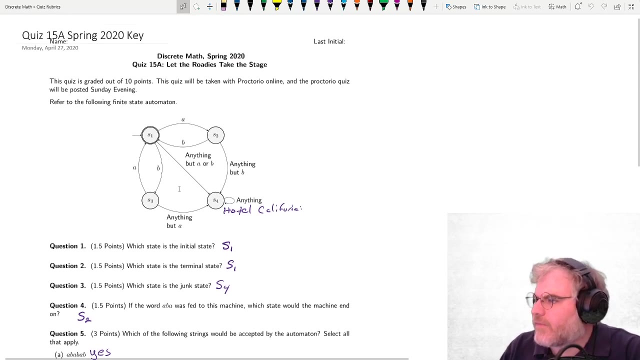 Yes, Are there any other questions? Okay, So let's look at this very quick. Let's let me see here How could I open this up. A couple things. One: I made an announcement. Let me write some of this stuff down. 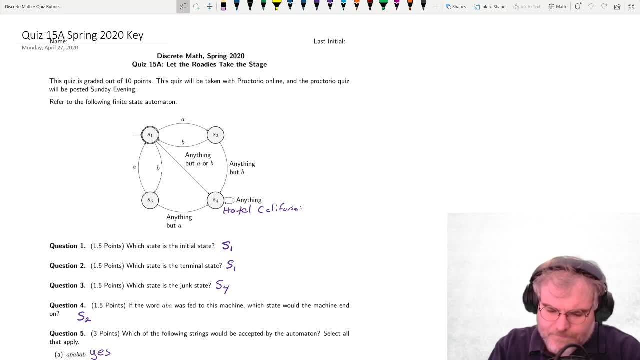 Um, And then my other announcement: blah, blah, blah, blah, blah, and then, at the end, Okay. So I want to go ahead and I want to talk about, um, a couple of announcements. One: I made an announcement that said: if you're going to send me stuff, please don't use Canvas. 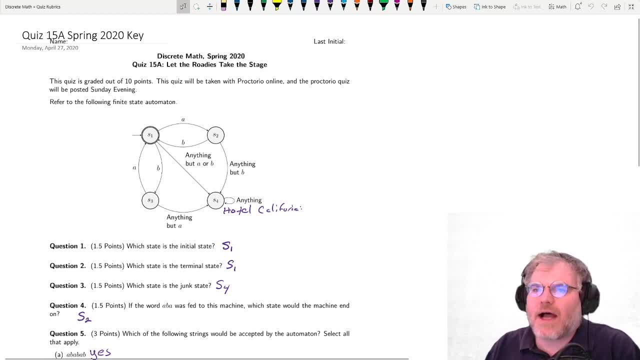 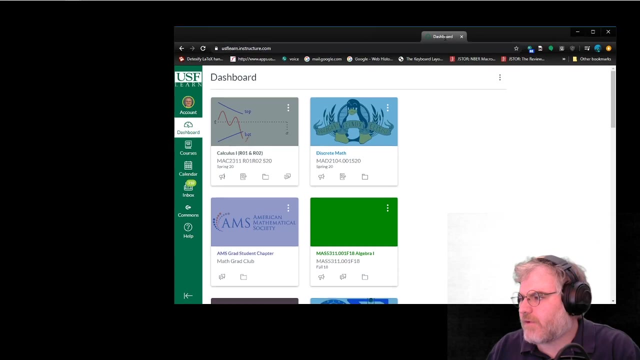 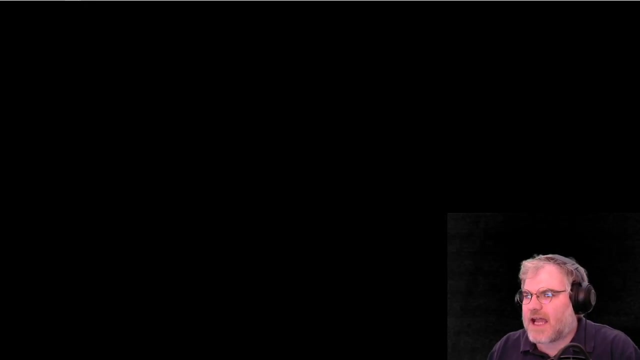 Canvas is great, It's wonderful, But you know, the problem is that I am literally on every calculus Canvas. Okay, So my inbox for my Canvas is absolutely useless, Right, It's got 318 messages or 10 messages or whatever it is now, and I cleaned this thing out a few days ago. 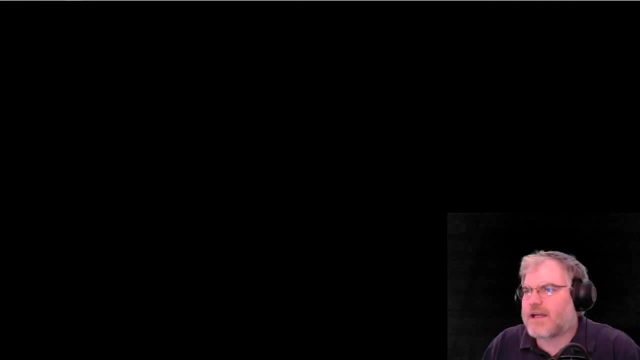 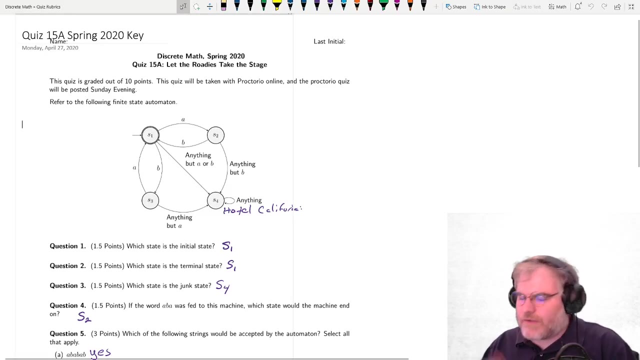 All right, It's absolutely useless. There are 1,000 Calculus. There are 1,000 Calculus students sending me messages- literally 1,000 of them, and I can't possibly. I have a filter, I can't use the inbox on there. 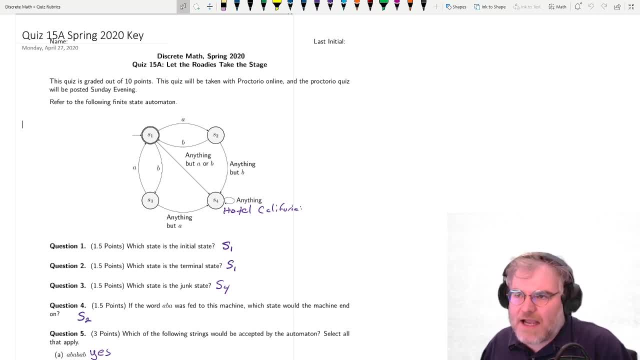 I have a. they go to my email. I have a filter to filter out your messages, but Canvas' forwarding thing is a little buggy. The other problem is that I can't forward if you send me work. I can't forward that work to graders through Canvas. 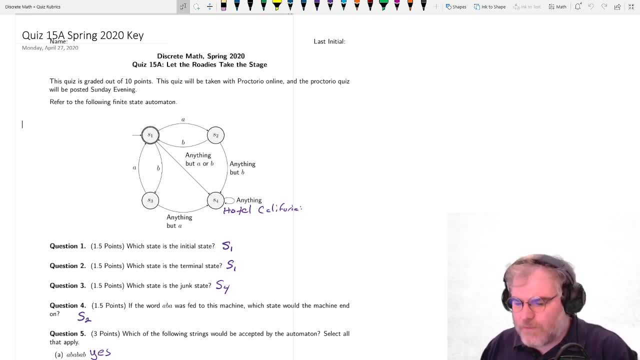 Okay, So you really need to send me. if you're, especially if you're sending me work, Um, If you want to get in touch with me, I can send you a message. I can send you a message. I can send you a message. 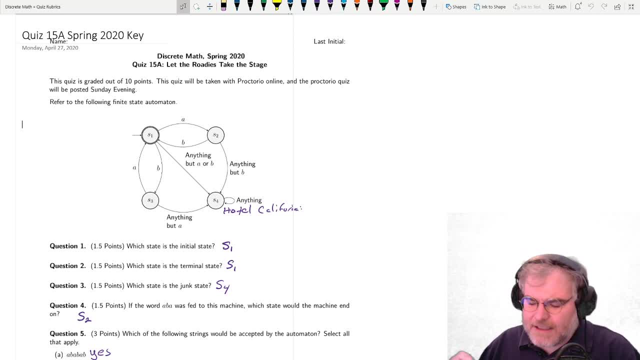 If you want to get in touch with me, especially if it's urgent, send me a Discord chat. If what you want to do is you've got old work that I've said you could submit, or something like that, please send it to me via email, because then I can forward it to the grader um and the appropriate grader for that assignment, because I have a list. 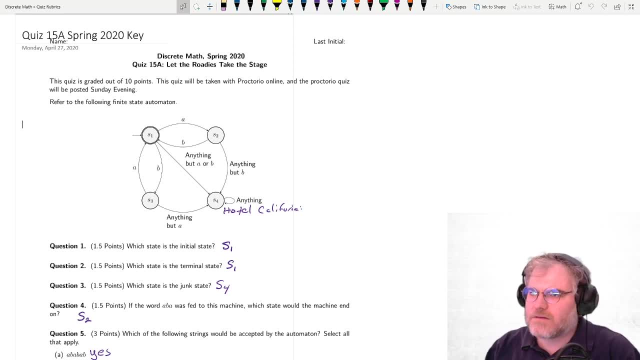 Are there any questions about that? Okay, So that was the first announcement, Um. The second announcement is: remember that the test is during class time On four. Um. Test four is during class time on Wednesday. Um, Now, just like last time, there will be um. 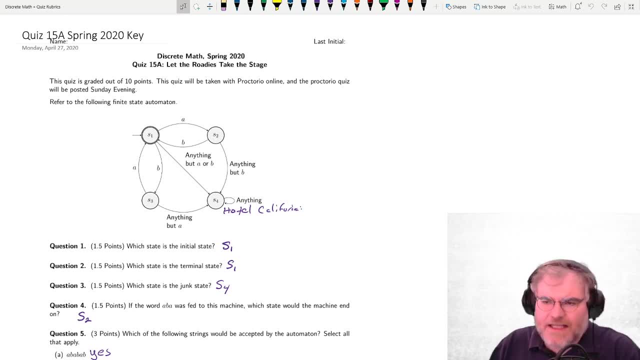 There will be. uh, We're going to jump on Discord, just like last time. We're going to use the phones. If there are issues, I'm going to have TAs with me. If there's an issue, we're going to deal with it then. 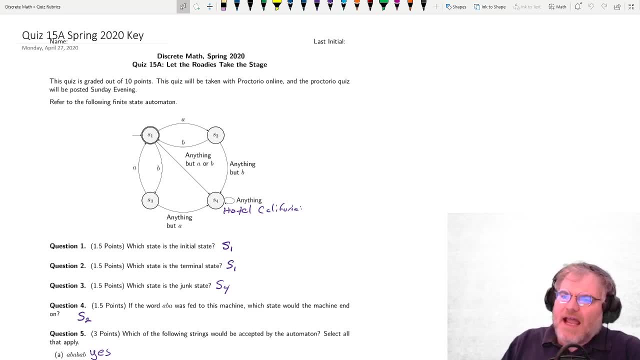 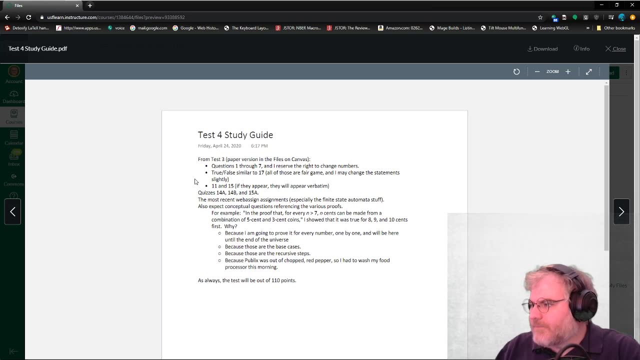 Uh, Does anyone have any questions about that? And I put up. There was a question about The study guide. The study guide is posted. It's right here. Um The Uh, I told you about the true-false thing. 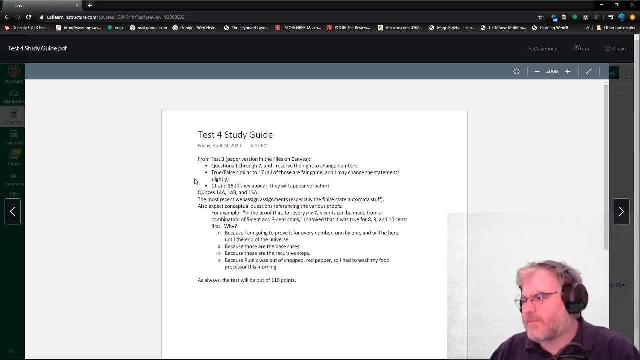 Uh, The test will be out of 110 points. People were asking: is it going to be mostly old stuff? Eh, Probably 60-40, 50-50.. Uh, Test three was really 50-50 anyway. Um. 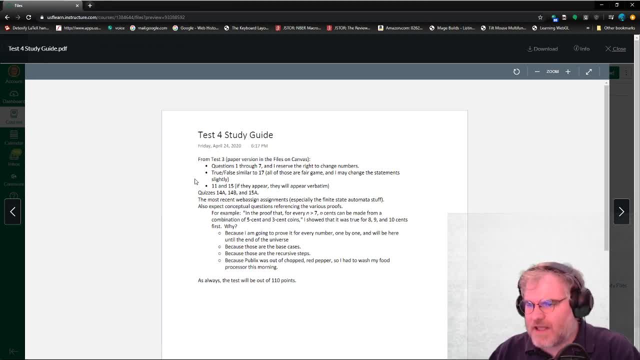 There's not as much material because there's only uh Two and a half weeks of class represented And I used one of those To go over stuff that you missed, One of the quizzes to go over stuff that you missed On test three. 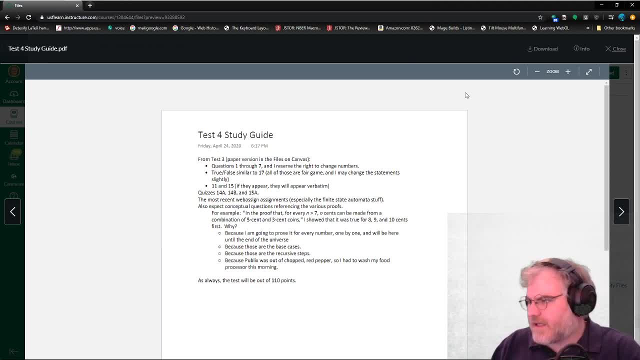 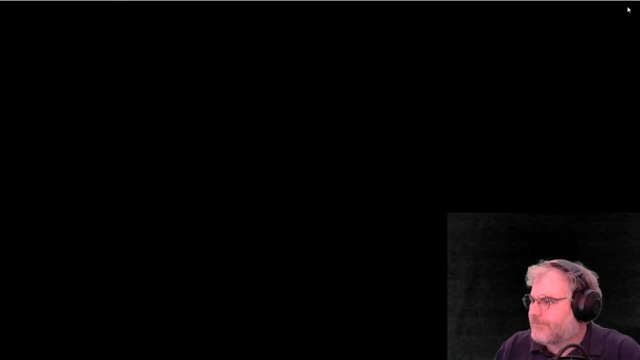 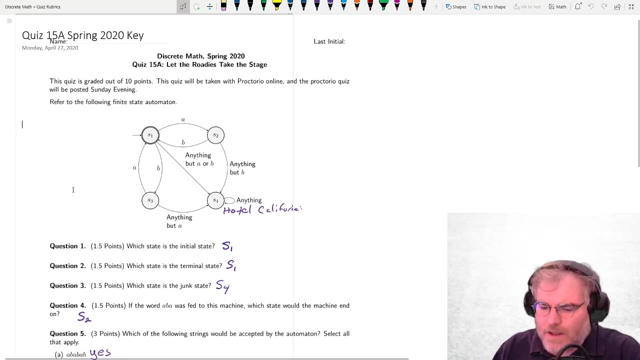 So, But today's lecture is on the test. Uh, So there will be questions about today's lecture on the test. Are there any other questions about that? Okay, Okay, So, Yes, Test store four starts at 3.30pm. 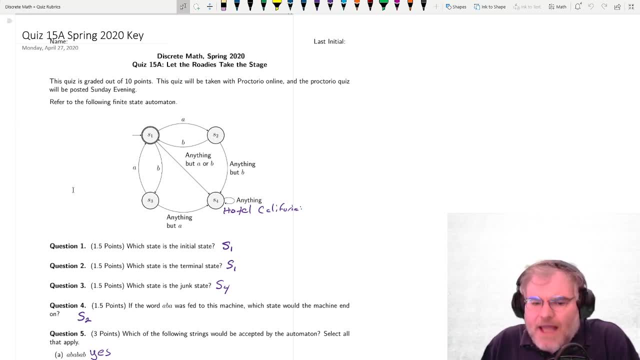 In class time. it is the last test, Um. I am not allowed to have tests on Friday Because of the Um, Because of the Uh Fact that it's a reading day, So we have to do it on Wednesday. 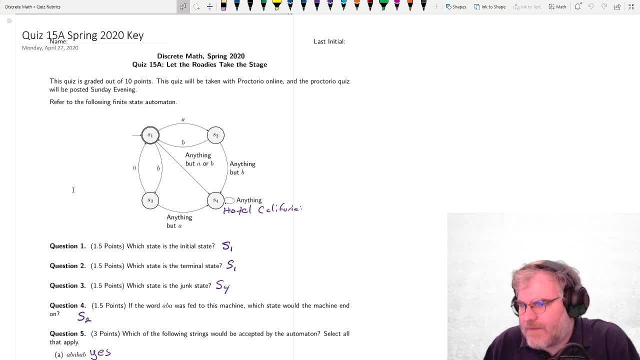 Uh, Not on Friday, And we can't do it during exam week Because we actually do have a final for this class. that's optional, Okay, First thing we want to talk about: Uh, Um, What proofs am I talking about? 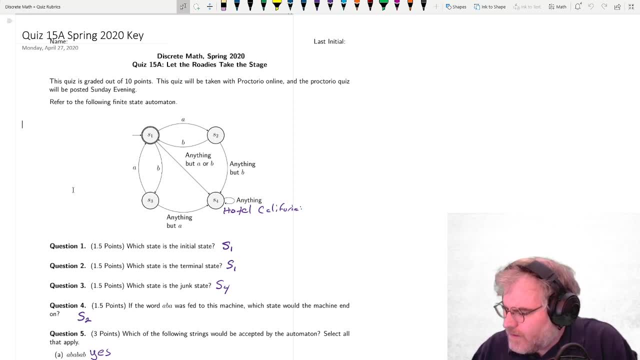 Um, I'm talking about the Um, I'm talking about the stuff that Like Um, This one, The halting problem, Um, Right, I got this move to zero, type thing. I can ask you one of those? 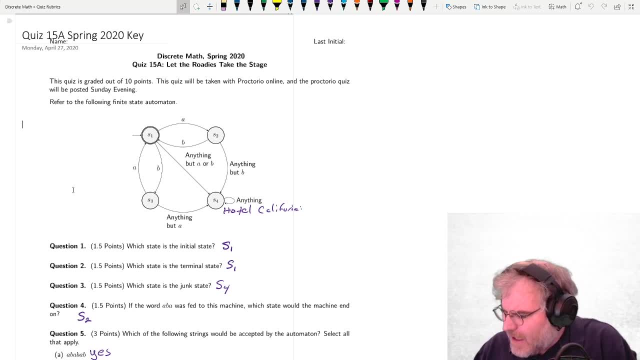 If I run check halt on something Like I did on the thing Um, The halting problems are good proof that I can ask you questions from True, false ones. Uh, I wouldn't ask the Tower of Hanoi, But I might ask something like this: 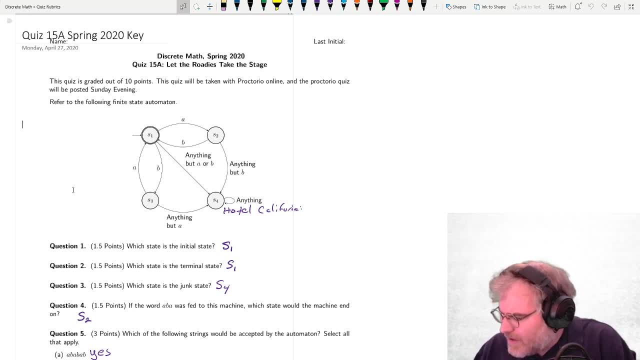 Um Uh. So read and try to understand this. I might give you some recursive function, And I did one. Um Uh Uh, This day was a write off because you didn't like it. Um, Oh, Every positive integer is: 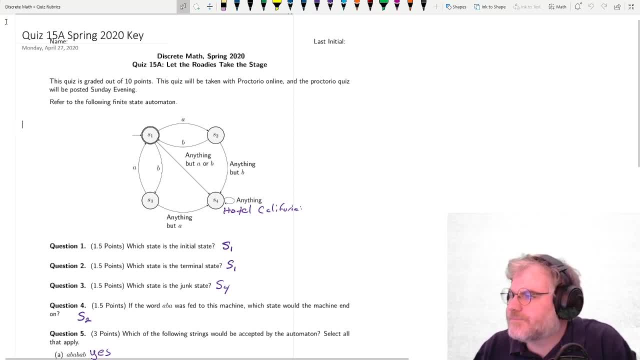 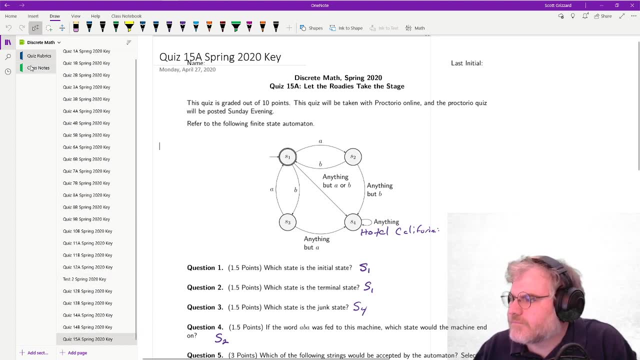 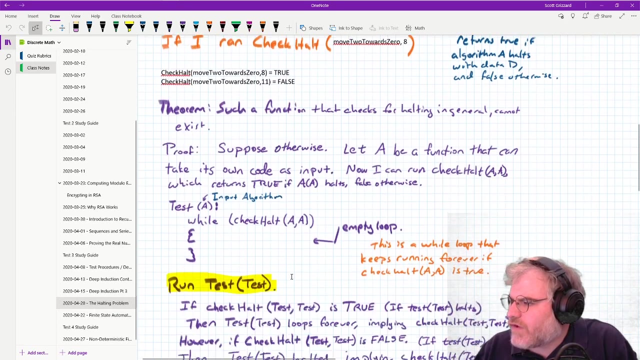 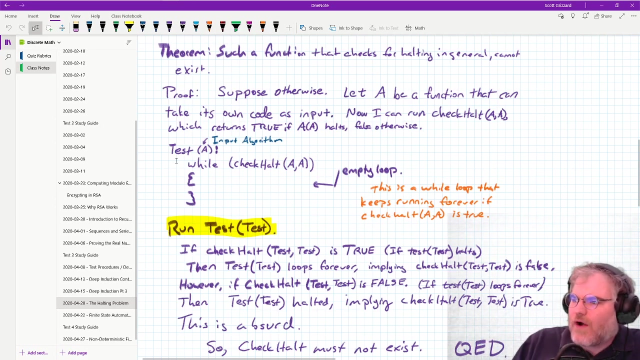 This is a good one, So, Um, Hmm, So here we go. I have this check halt stuff. I have this question right here, The ask, and like: what is test? I could give you an easy, true, false one. Um, 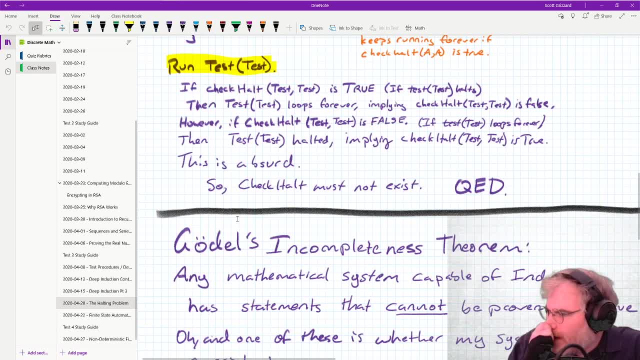 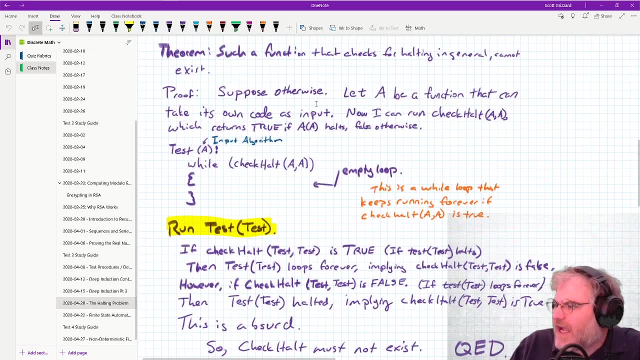 Like this: Okay, Um, I could give you something like this, Not that The Goldelstern is not good for this. I can give you something like this: Like I tell you that test day is wild, not check halt, Or something like that. 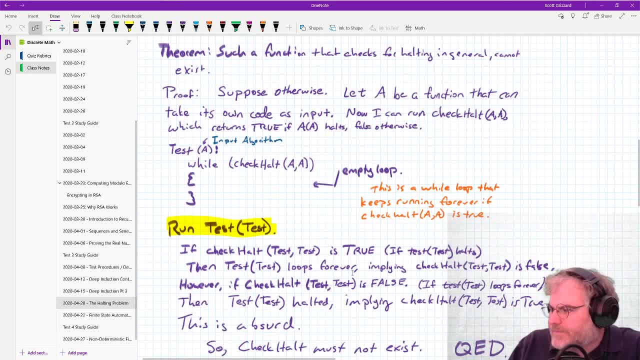 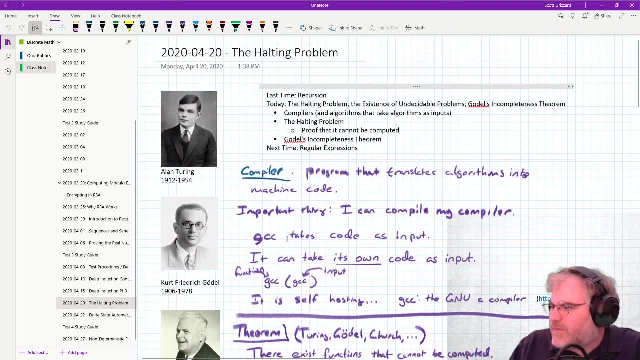 Um, I could ask you something like this: Um, Uh, You know how you get the contradiction, That sort of thing. So reading and understanding these proofs is important. Um, I could ask you about the. I could give you an idea about a machine taking its own code. 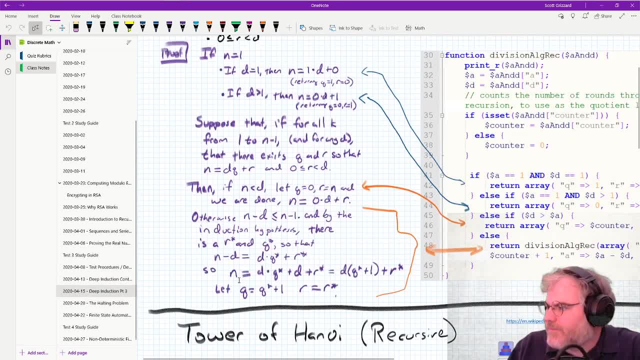 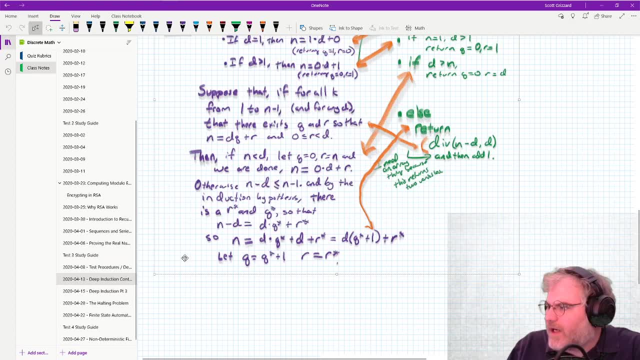 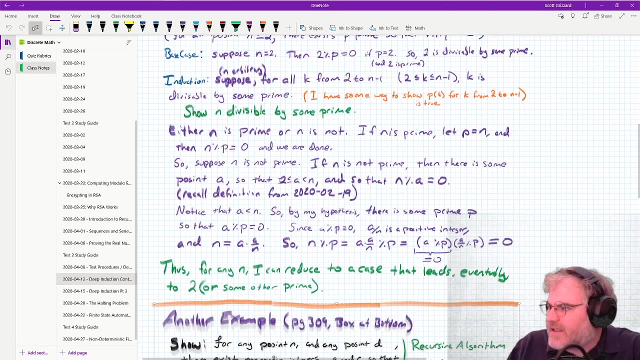 As an algorithm, And I could compare that to a recursive function. Um, This I like it, But you know it doesn't work very well. Uh, This is good, The fact that I can induct, And I find that there's a positive integer. 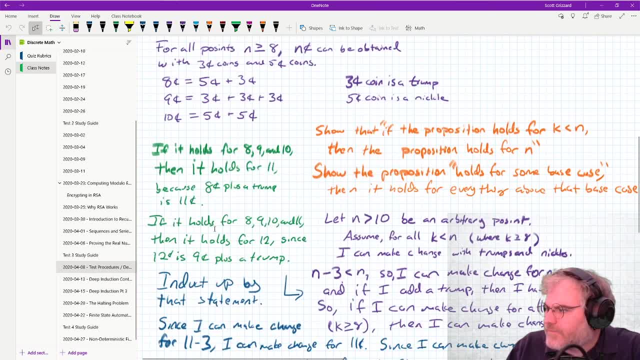 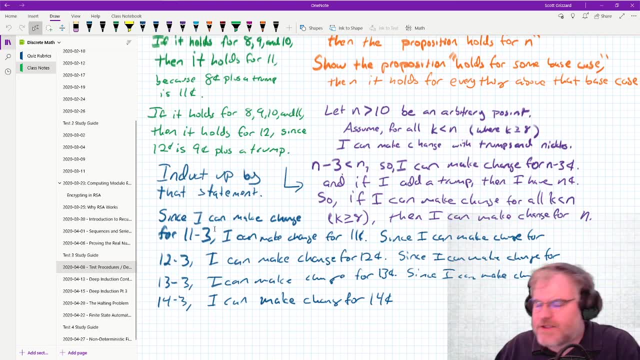 Um, Um, Yeah, So those sorts of things are nice proofs. So those will be the proofy questions. They'll be true, false, multiple choice. I'm not trying to trip you up on them, Um, Uh, But the. 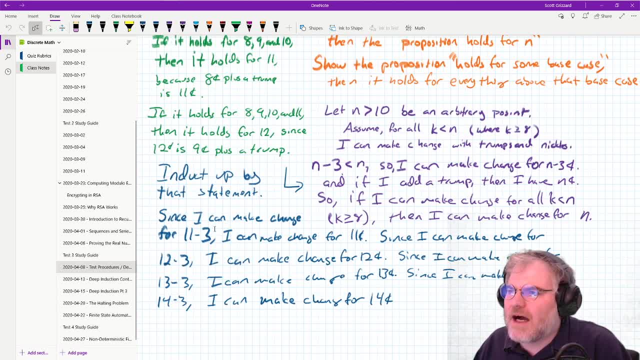 Um, And we are done with quizzes. Yes, Um, So that's the kind of things that it'll look like. All right, Any other questions On that? All right, If you have more questions, I'm more than happy to do it. 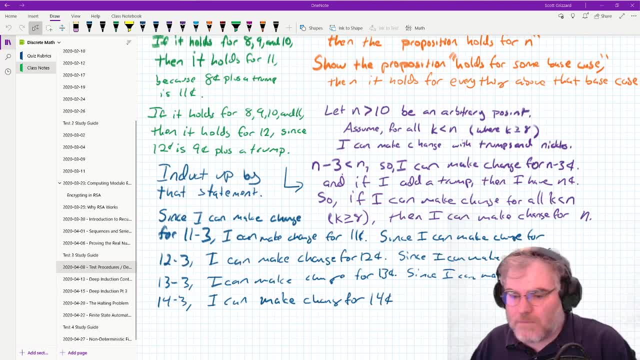 I will have extended office hours tomorrow, Which I don't normally do, But I am going to have extended office hours, Uh, Tomorrow For you to ask questions. I'll be happy to jump on Discord, Twitch, Whatever, Um, To try to talk about some of these issues. 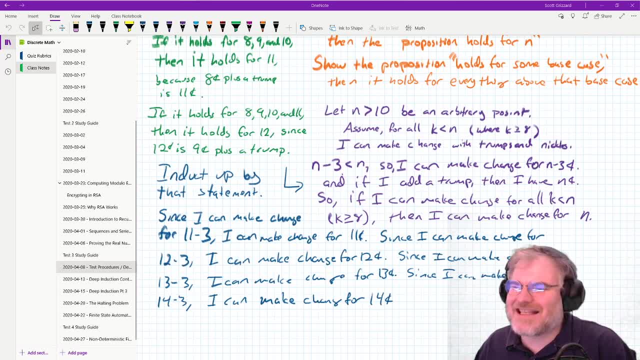 If you've got specific questions. I think it's going to be more like test three Than anything else. Okay, It's going to be Lots of multiple choice, Some multiple selection, Some You know Various, Uh, Some true, false. 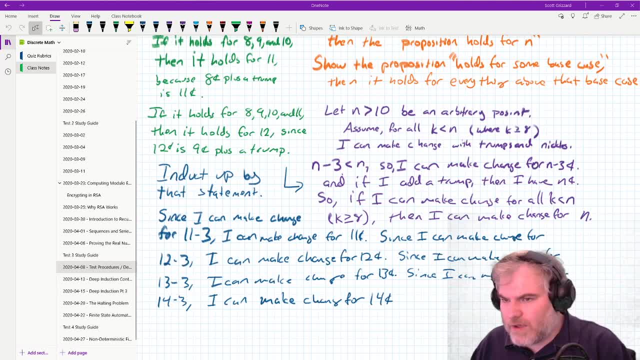 Um, Some fill in the blank, But it's going to be very straightforward. Um, Most of the questions are going to come for the quiz Quizzes. Um, You know, I might change some numbers, Um, If the quizzes. 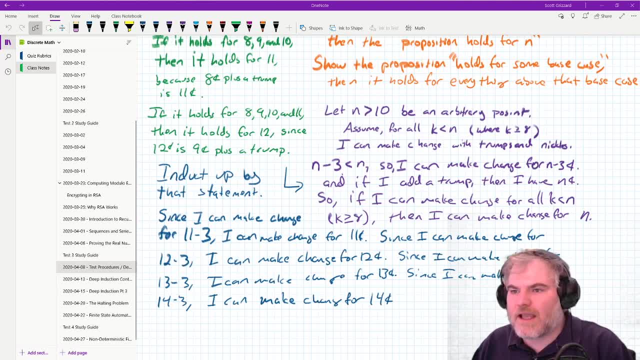 If they're not coming from the quizzes. I'm going to try to limit the number of points Like Uh, That The non-quiz questions come from. So If you're prepared for the quizzes, You're going to do fine. 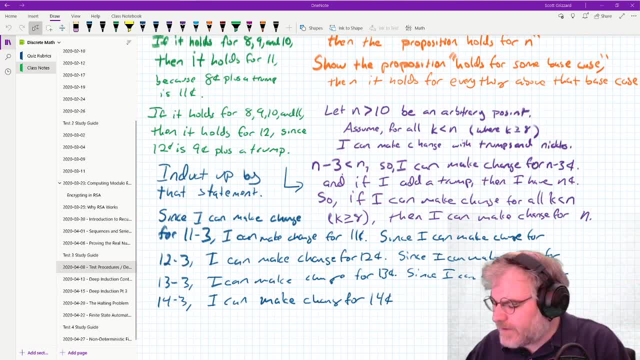 Are there any more questions about that? Okay, So let me start talking about stuff, Because people are going to ask me test questions all day And I really do want to talk about non-deterministic FSAs And I want to talk about compliments. 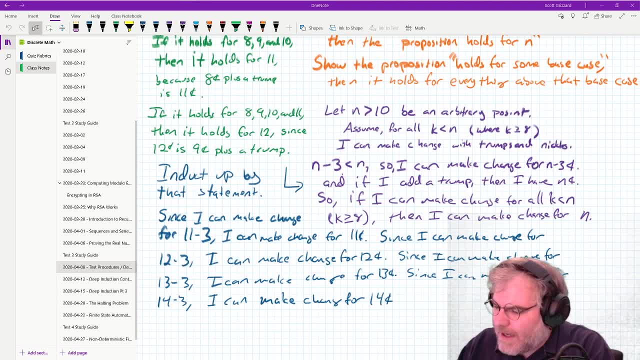 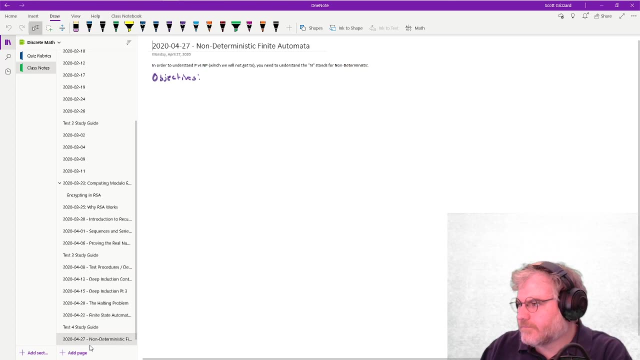 So today's objective is to talk about: Okay, So, objectives for today. Um, The first one. Um, The first one is to define and give examples of non-deterministic FSAs. Okay, FSA, Uh, I actually can't do that very well. 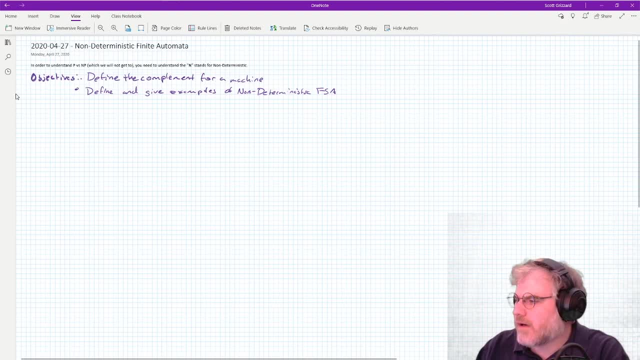 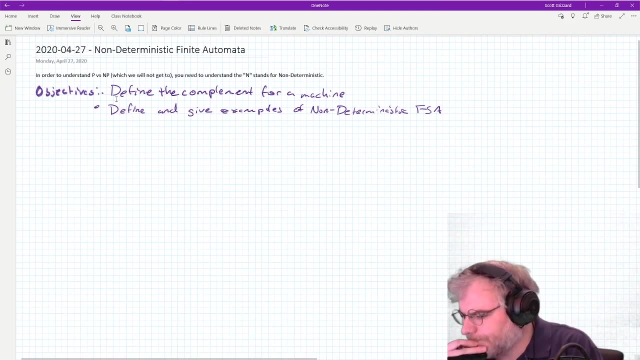 Can I Do this Alright? Okay, Okay, so, Um, There's a question about: Uh. So There's a question about A machine taking its own code. Think of it more like a function's input is the letters. 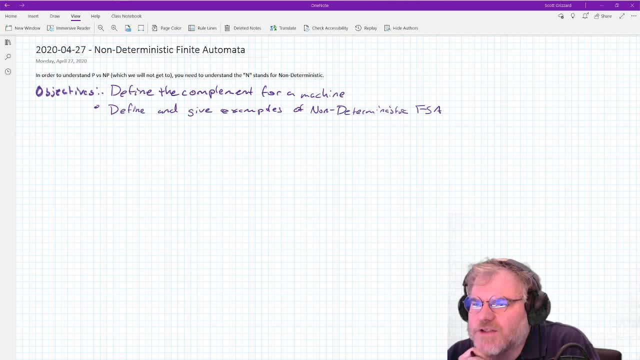 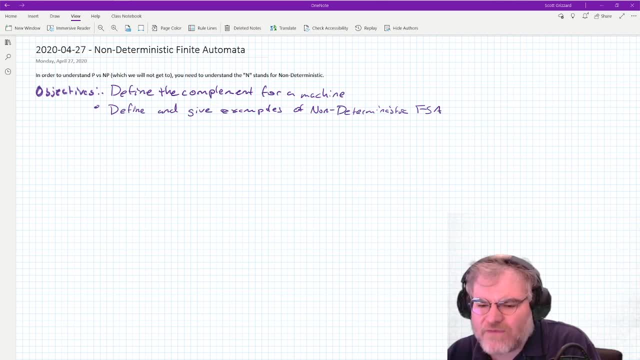 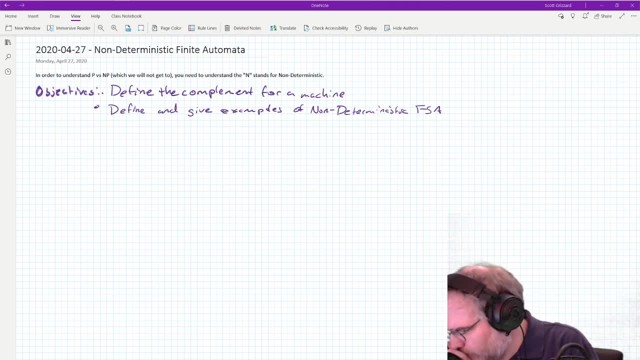 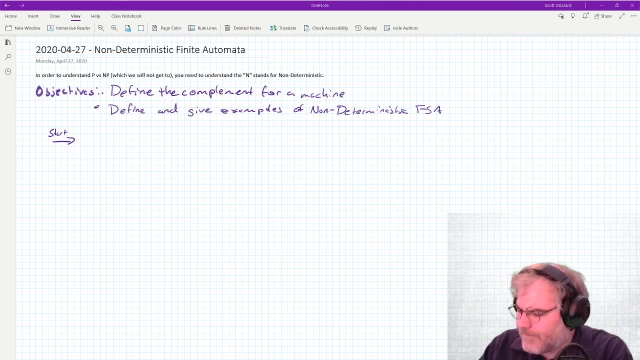 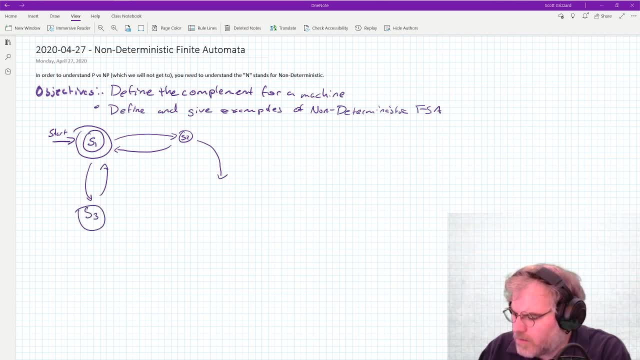 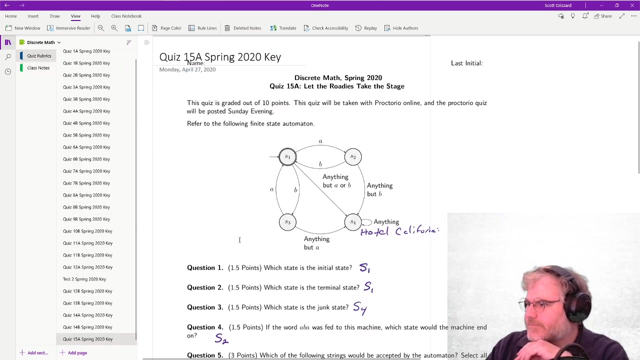 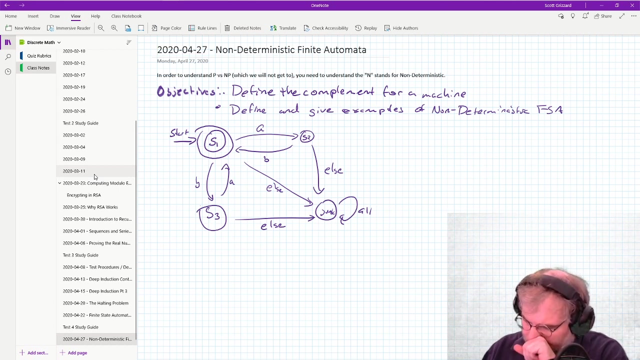 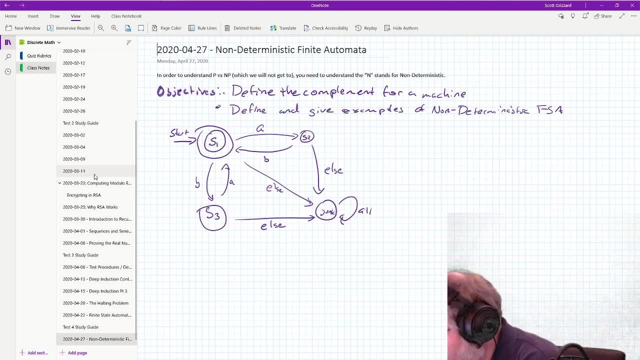 dude this word. what is? what would be a description of this machine? by the way this machine takes, let's see it. takes, start the grouping a B, which is not to be. they know, not the, not the print, not the class, but the actual a B together, star and does. 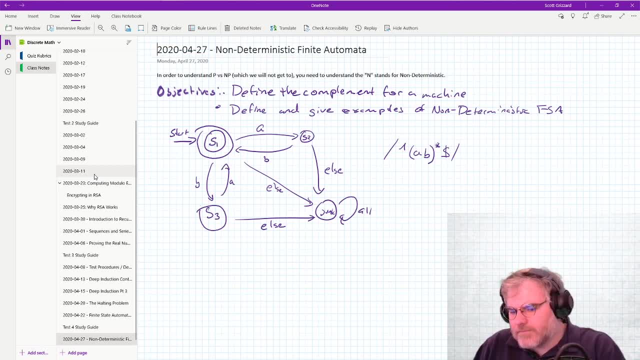 everyone agree with that? one to five. how do we feel about that? that the connection between those two things is to be ready. so you, you, you, you, Okay. So there's a question in chat. does every regular expression need to be enclosed with that? 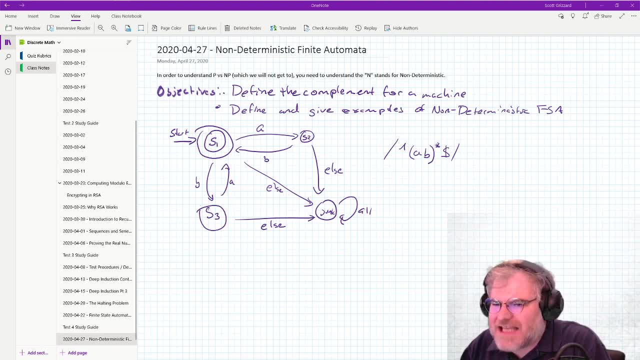 In the book. no, The book is using generic regular expressions. I'm actually using- I'm using irregular expressions the way PHP uses regular expressions, because I want the idea that this is code to stay together. That's a very good question. 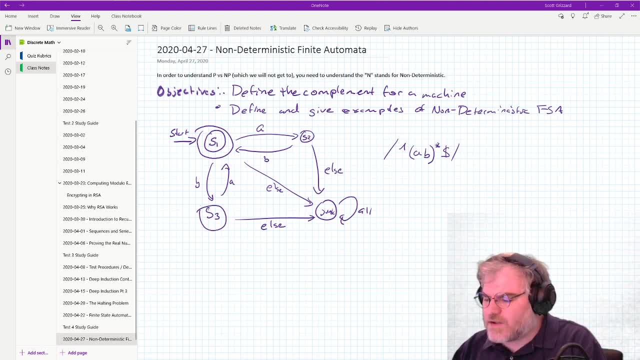 This end string. we're actually going to talk about ones that don't have start and finish positions. So this is the start position and that's the finish position. This is the start and that dollar sign is the finish. But I'm going to get in today one of the points of 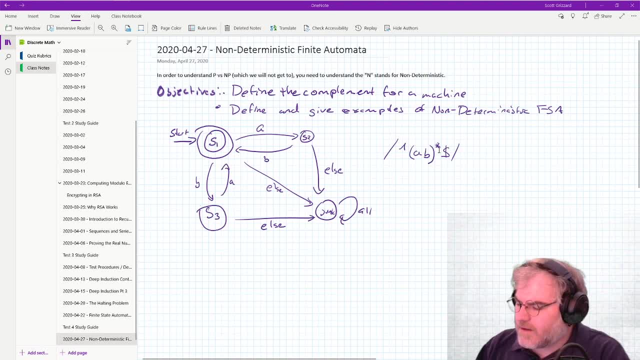 non-deterministic FSAs is getting rid of these things. when I want to match anything in the language, All right, This is called the language. Now can I write a finite state automata that would accept anything but that? So how could I do that? 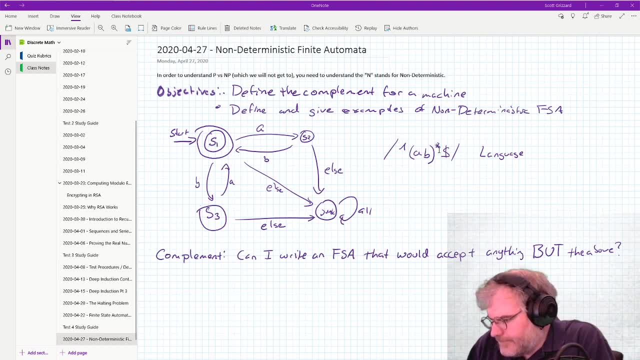 Well, like this. Now, what I'm going to do is: everywhere at the initial states are the same, but I don't want to accept anything that this machine accepted. So that means getting rid of S1 as a finite state automata. So I'm going to get rid of S1 as a finite state automata. 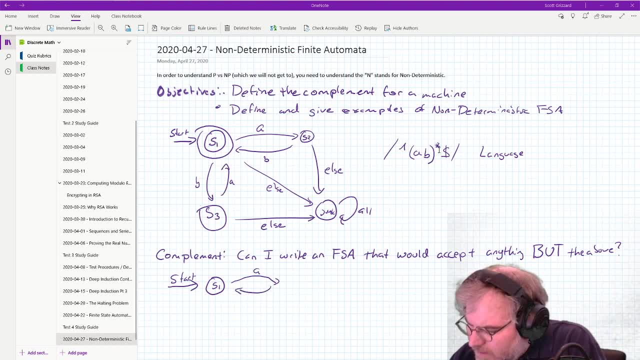 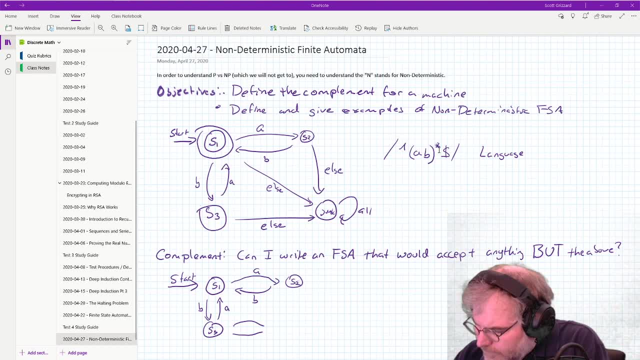 It's not a majority or part of theりますneedling pastors parameters. So the problem it fully does is it's an astonishing number of blocks, And these two blocks- they're all- are called the 16-megayner elementary schools. But I say rather contractually. So, first of all, which determines this says: well, it's not cookie. All characters simply ought to belong to somebody else. Fella like having to type your own lemongrass, Always and always. 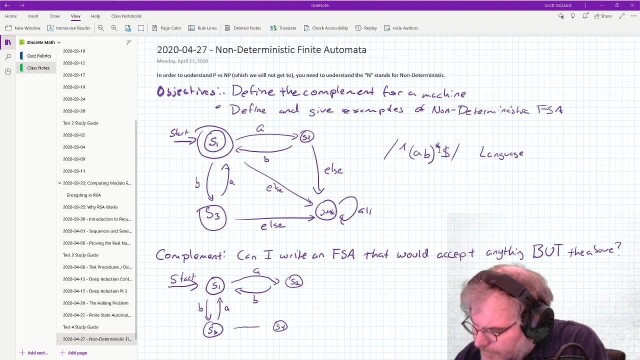 everyone on board with that. how do we feel about that? I want to ignore at. how do we feel about that? one to five, okay, and then what I want to do is I want to accept every state that this thing would have rejected. so now I don't really have a junk state, because now I'm 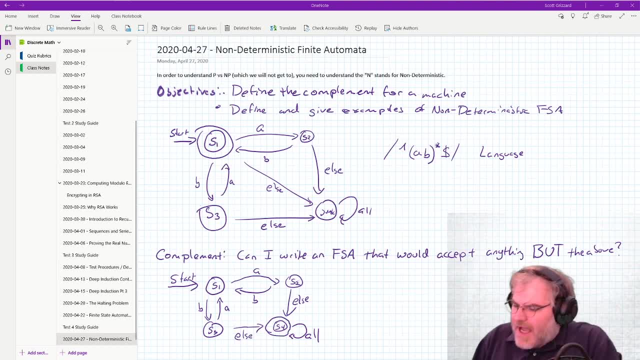 going to accept it all these states? is everyone on board with that? this thing right here will accept see. this thing will accept: see. yes, it needed that line. this thing will accept: see. this thing will accept anything as long as it's not that not accepted by the first state machine. 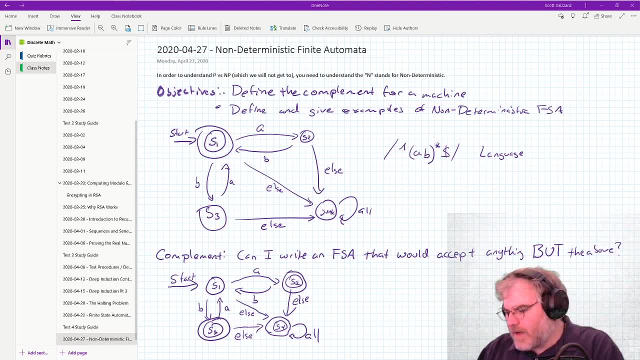 right, yes, so my junk state is no longer a junk state at all, is it now? it's a terminal state, so as to. so as s3, so as s1, I'm sorry, not s1, everything, but s1 is now terminal now, because every regular expression 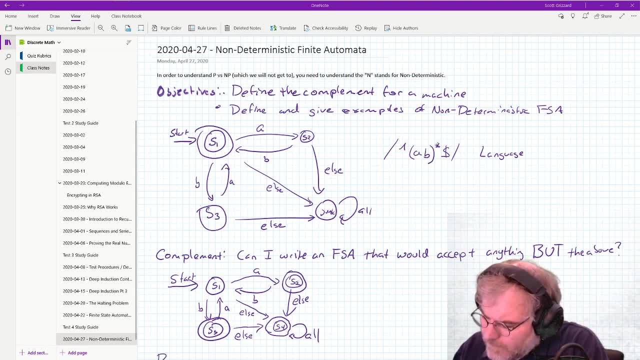 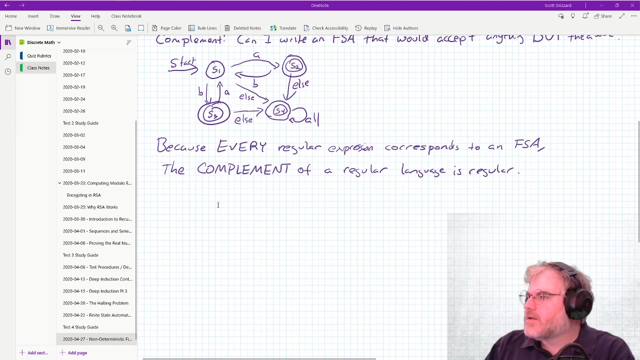 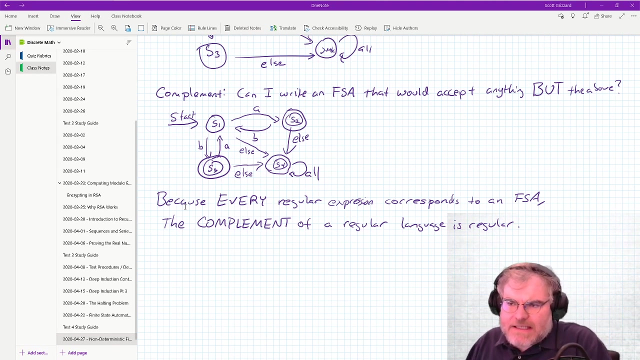 you, you, you, you, you, you, you. And I know I need to move it down, Because every regular expression corresponds to an FSA. the complement of a regular language is itself regular, And this is actually weird. Okay, This is not true for classes in general. 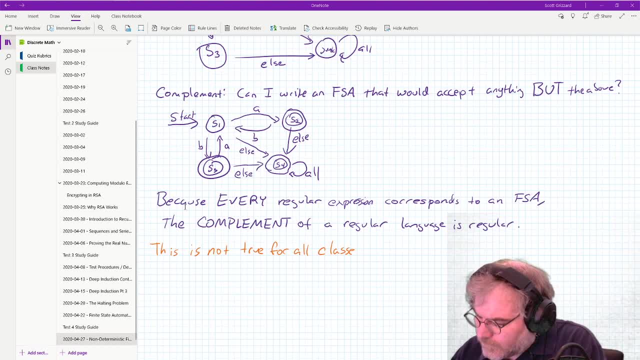 Okay, This is something strange about regular languages, Okay, But okay, that's one thing. So you're going to see complement problems like this in other things, Like if you're talking about the complement of an NP problem or the complement of a polynomial type problem. 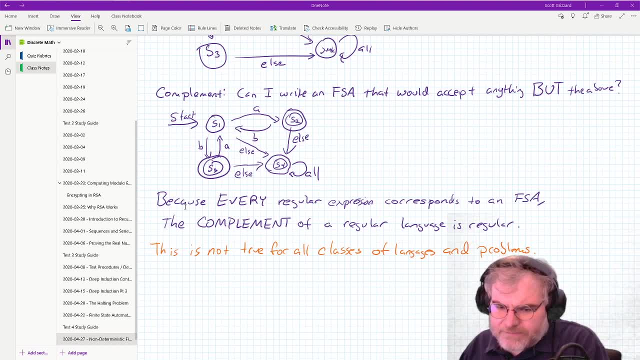 or the complement of a exponential problem. Okay, And a language is regular if it corresponds to a regular expression. Technically, it would be determined by a regular thing. Okay, How do we feel about that? one to five, That's a good question. 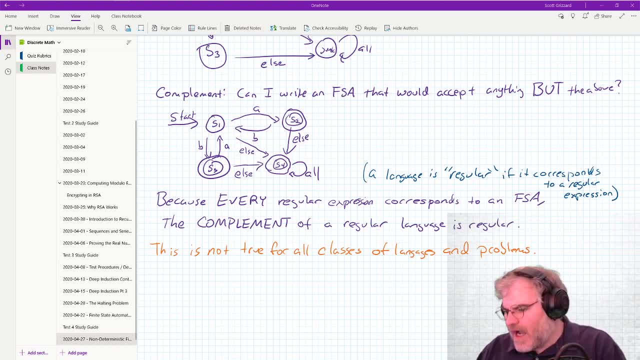 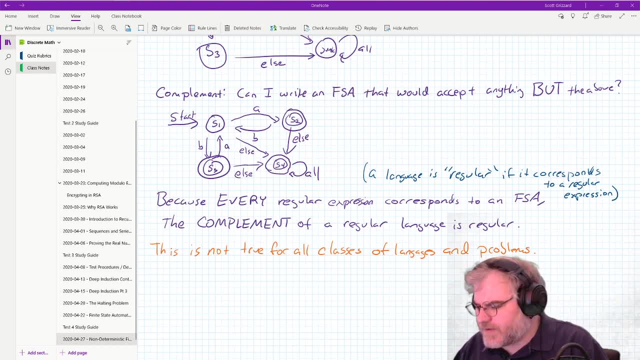 And again, that's kind of a weird thing about regular expressions in these FSAs: They're very nice, Okay, All right, All right, Now, Now, Now, Now, Now, Now. we had a question about this orbit. 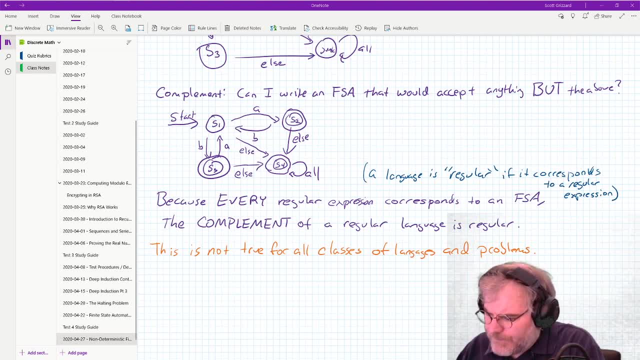 And we had some other questions about these regular expressions. Okay, So let's go in. Let's talk about non-deterministic machines, And this goes into that. you know all of these various things. Okay, So let's look at one of the ones we had from last time. 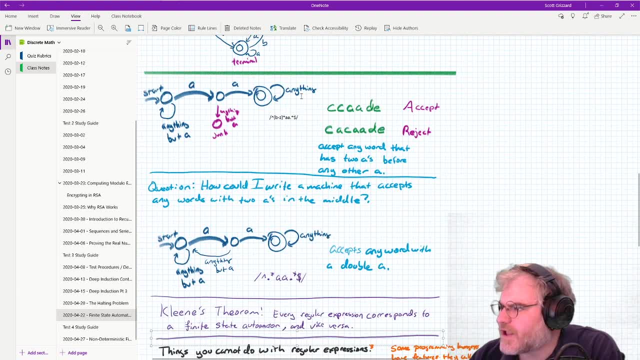 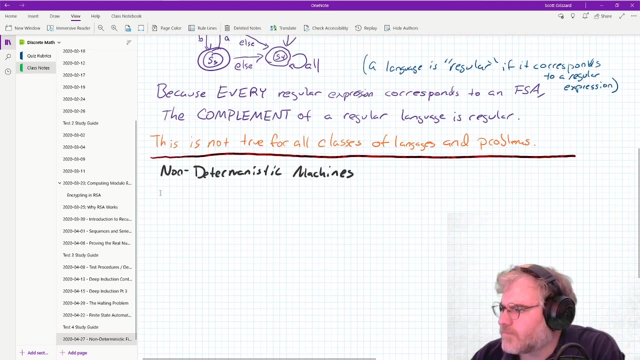 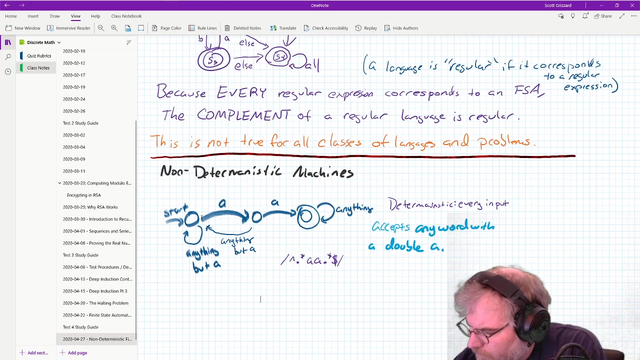 Remember, not that machine, that machine, not that one. Remember this machine Here. This was a machine that accepts any word with a double A in it, right? This is called deterministic. This is called deterministic. This is a machine that accepts any word with a double A in it, right? 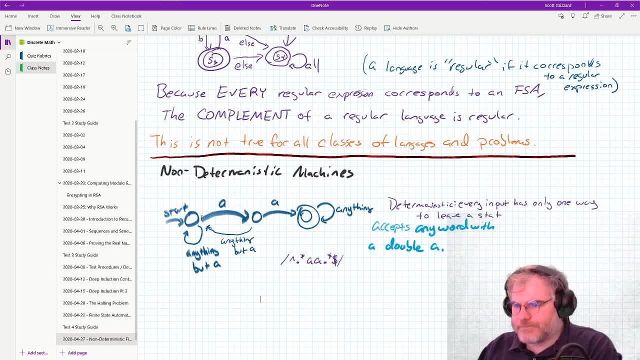 Okay, Every output only has one way to leave a state. Okay, So this one, no matter what it is. if this is A, if I'm at A, I'm going to have to leave a state. If I'm at A, I'm going to have to leave a state. 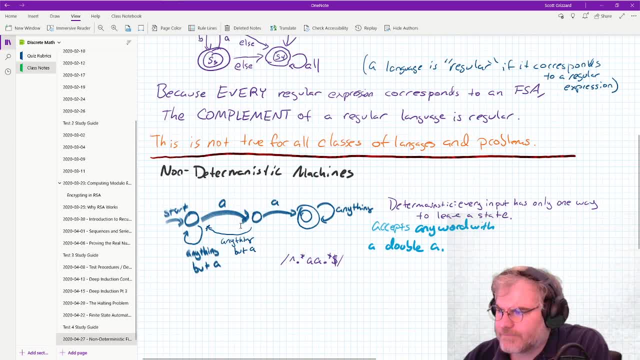 If I'm at A, I'm going to have to leave a state. If I'm at A, it's going here And then it's going here, and then it comes back right And anything. after A went back to the starting state. 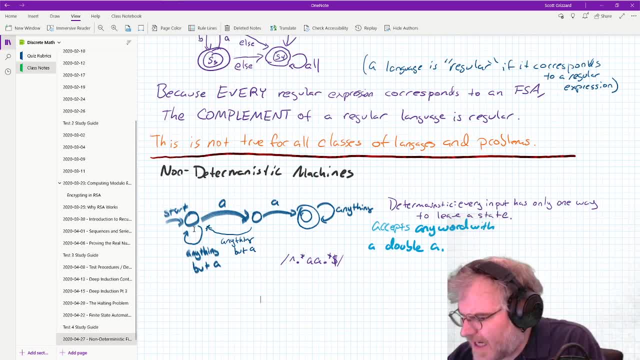 I can also draw that. let's look at another machine that does the exact same thing, But this one's going to be non-deterministic. But this one's going to be non-deterministic. But this machine non-deterministic is that A can go one of two places. 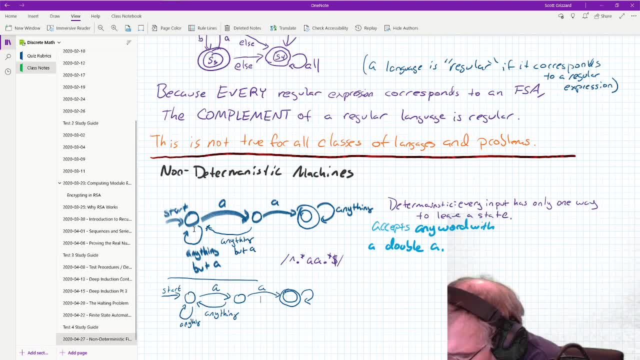 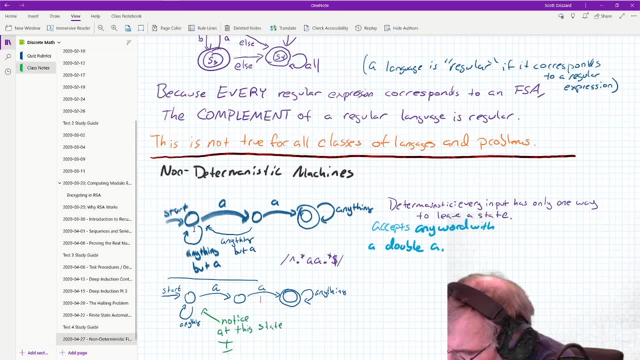 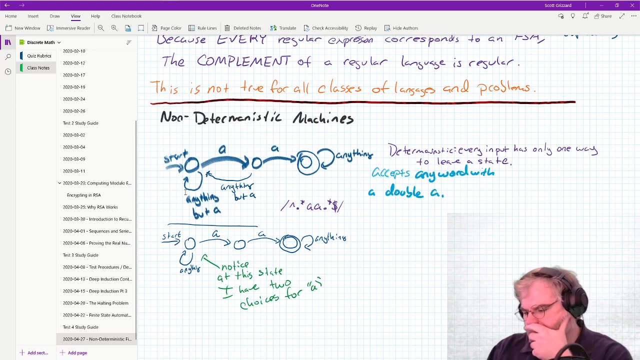 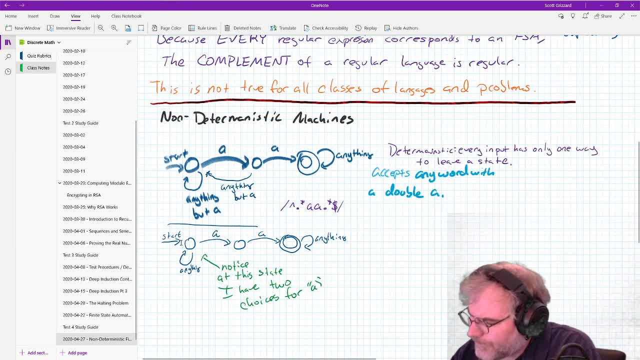 So let's trace the word here. Okay, here, if I want to trace the word, let's do this And let me label some states here. Okay, so if I wanted to trace this input, what would happen? Okay, so here I would go: S1 to S2 to S1.. 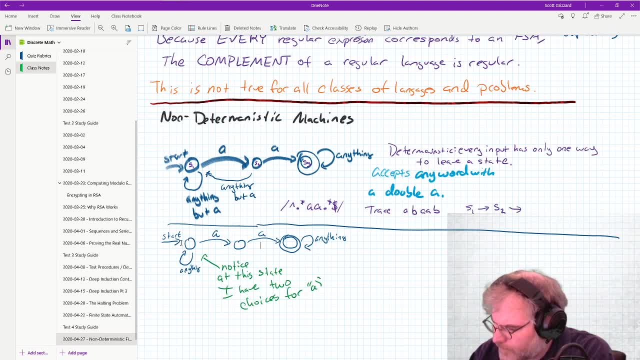 Okay, so here I would go S1 to S2, to S1.. Back to S2. And then to S3.. And then to S3.. Okay, so does everyone see that? Okay, How do we feel about that trace 1 to 5?? 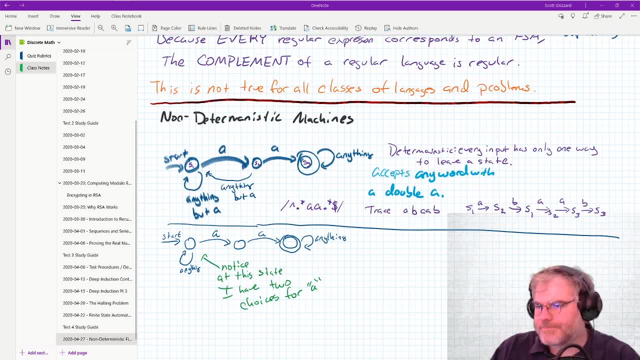 So this is on the trace. This one was on the complement. Okay, Let's trace this one. So I started A. Okay, Then I went S1 to S2 to S3.. Okay, Okay, Now I've got two choices. 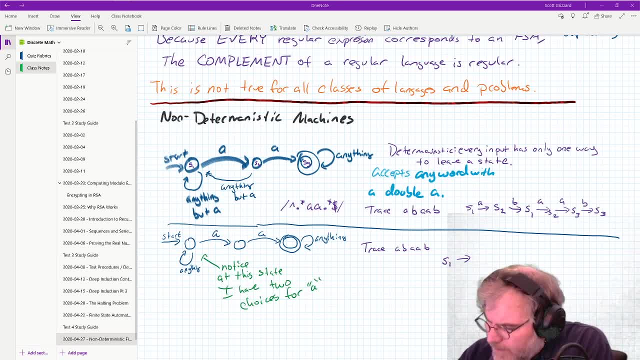 I could go across A, from S1 to S2.. Or I could stay at S1.. Okay, I don't really have a junk state pointed, but that's the point I wind up with junk. however, I could have also gone from S1 back to S1. 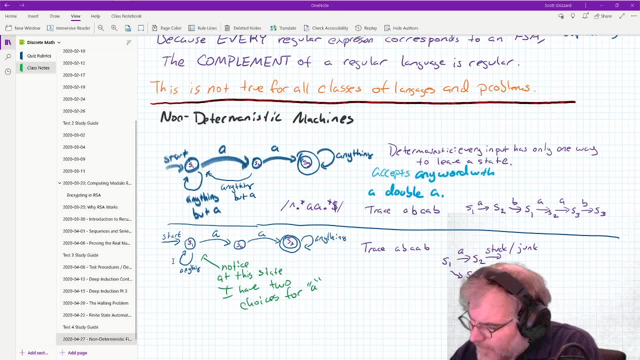 along the anything and then gone to S1 along with a B, then gone along the A to S2, then to S3, and then to S3 except, and then to S3 except and then to S3 except. how do you feel about that? 1 to 5. 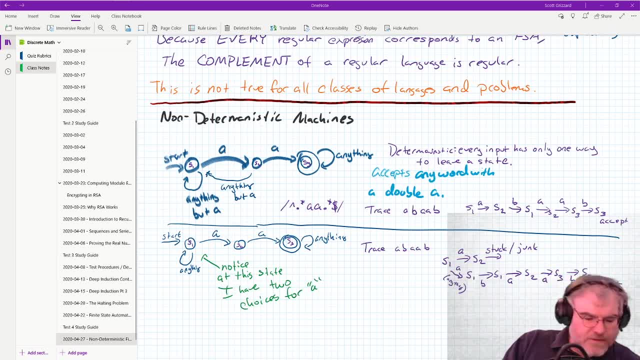 oops, I missed it again. and the key here is that they accept the same thing. yes, it's non-deterministic. okay, so as long as there's a potential path to a terminal state, it's considered accepted. now this gets us back to the question we had. 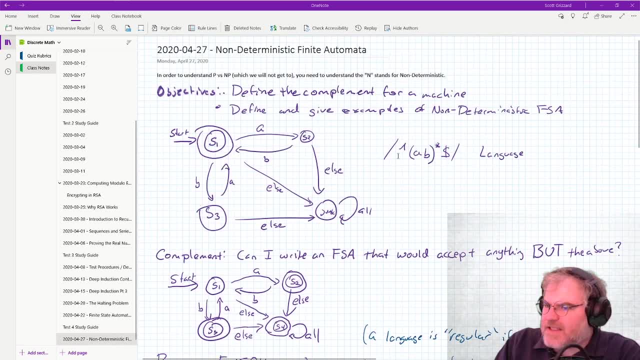 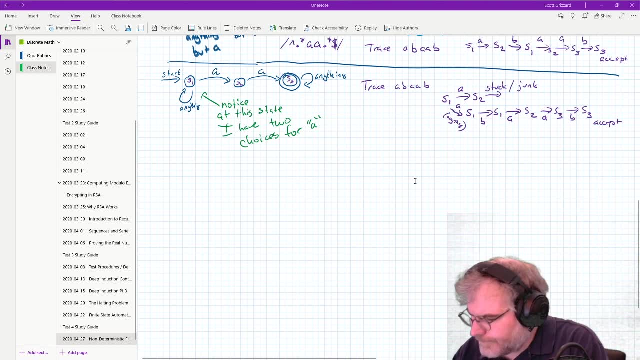 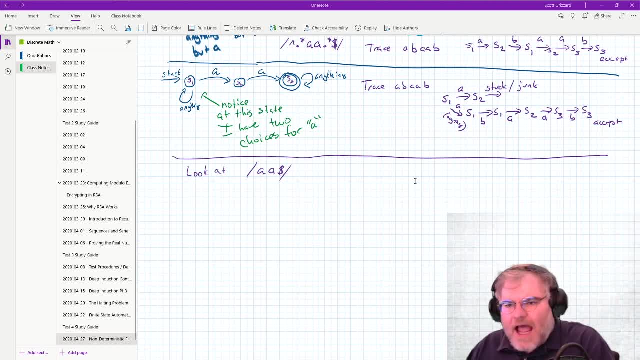 If I don't have a thing, but I do have a terminal, how can I write this language? Well, this is the same as saying the following: Right, So let's look at it. I know I want a state that's going to end. the thing has to end at a, an, a. 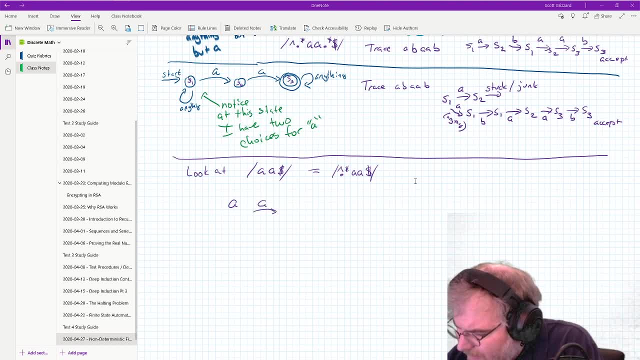 So, whatever it is, I'm going to have a terminal state here and I'm going to have a state with a on it. Sorry, Now here's my initial, And then I just have an anything here, And then I'm done. 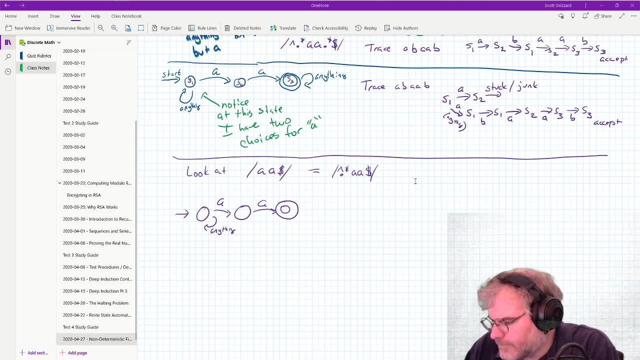 All right, I don't need to deal with the issue of curving a's in the middle here, because I don't care. right, I don't need the. if I wanted to do this with a deterministic FSA, right? If I wanted to do this with a deterministic machine, I would have to put here. 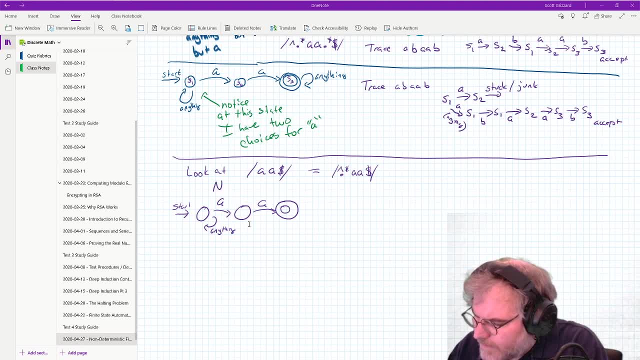 So this is the non, the a's And FSA here. If I wanted the deterministic finite state automata to do this, I'd have to do something similar, But I'd have to have one of these here. here, This would have to be. no, that's not an acceptor. 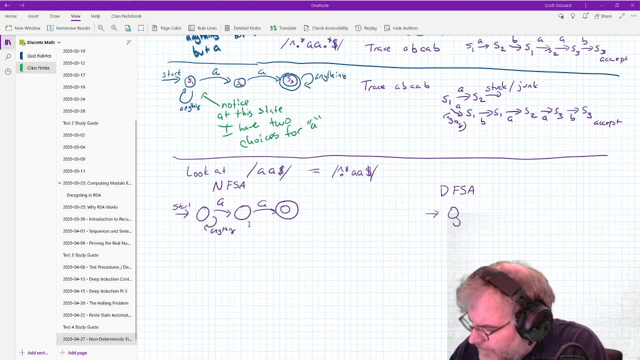 This would have to be anything but a. This would have to be Right. This is a. This would have to have a state back here: anything but a. All right, Here's an a. And then I've got this terminal state with all of these things here. 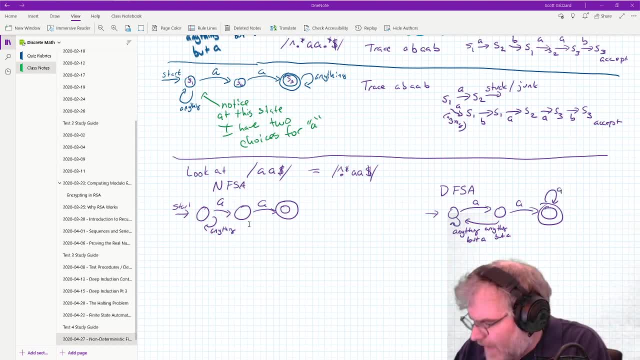 Here's an a. So if I keep punching up more a's, I'm fine, But if I don't keep punching up more a's, I have to go back to the beginning. How do we feel about that? one to five. 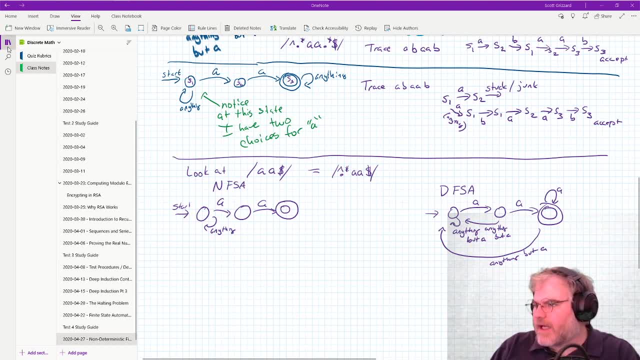 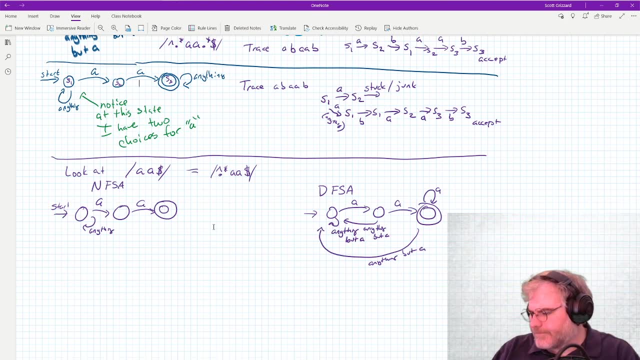 I've got a non-deterministic way of doing it, And then I've got a deterministic way of doing it. Okay, Okay, In fact. Okay Okay, the two languages are equivalent. anything i can do with an nfsa, i could actually do with a. 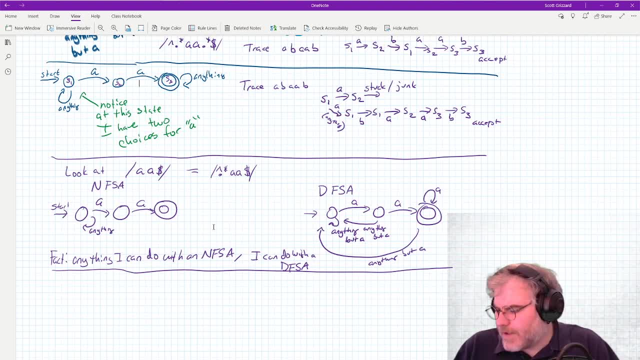 deterministic one. okay, i can build a deterministic one. i can build a deterministic finite state automata that corresponds to that non-deterministic finite state automata. indeed, there's an algorithm to use it. do it, you can find it online. okay, there's a nice algorithm that will convert. that will take one of these. 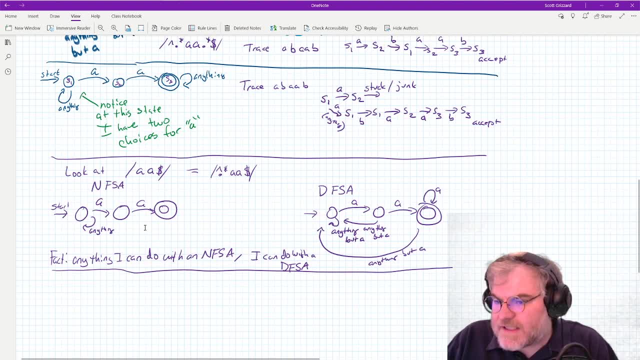 these automata here, uh, with all of its states and all of its arrows, and convert it to something of that form. how do we feel about this? one to five: there's a for every deterministic. there's a. there's a. there's a corresponding state automata that corresponds to that non-deterministic. 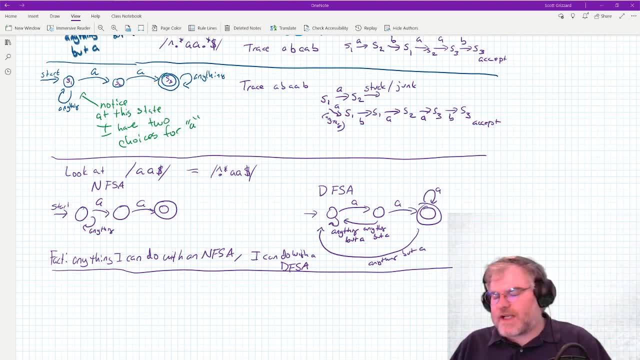 non-deterministic. i'm not going to prove it, i'm just going to do some examples. the proof involves an algorithm that's very long and nobody cares. um, i don't know why the, the polling is not. uh, did the robot hang? uh, hold on, let's see if the i think the. oh, there it was, then it went. sorry about that just as it. 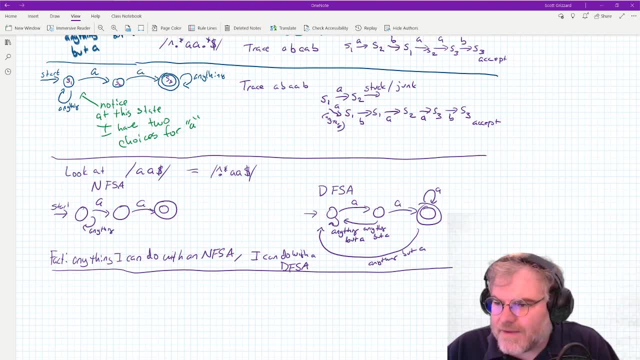 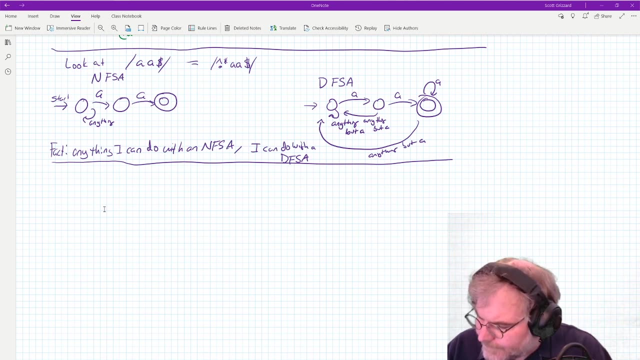 figured it out. i deleted it. uh, the bot hang. uh the bot hang. uh the bot hang. okay. okay, but, as i said, the nfsa is is simpler. but, as i said, the nfsa is is simpler. but, as i said, the nfsa is is simpler. now let's go into this thing. 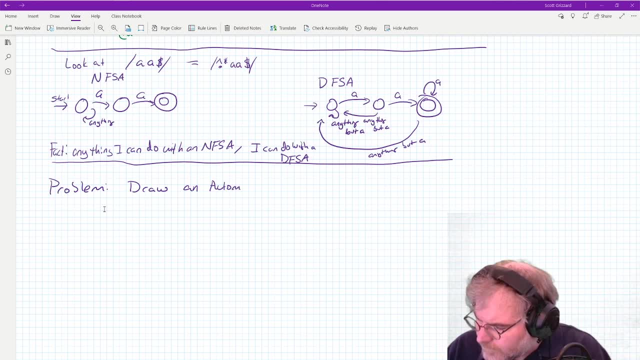 now, let's go into this thing now. let's go into this thing now. this is saying two a's. now this is saying two a's or two b's and the a dos is ok, just do that deal is in this one here. these� the string in a row, okay. 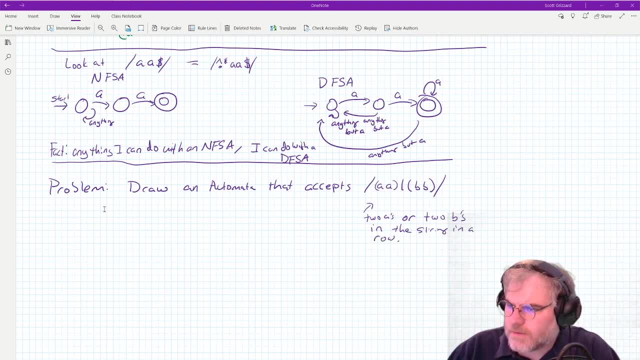 Okay, Okay, Answer your question. Is there an algorithm for converting FSA and regular expressions? for vice versa? Yeah, that's how Klein's theorem works. Klein's theorem works. If you want to actually read what Klein's theorem says, that's what it says. 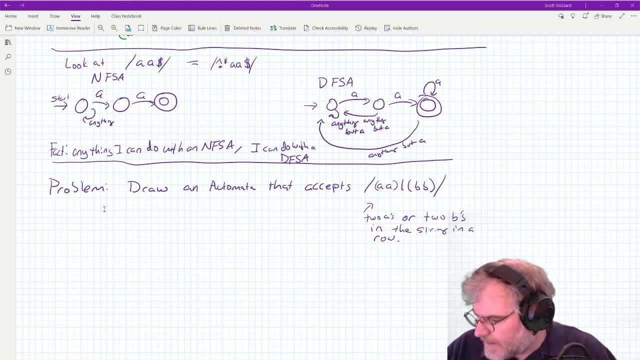 It's an algorithm for building the thing, All right. Well, how do I do this? Two ways or two B's in the middle of a word, All right. So the first thing I notice is I've got this state here. 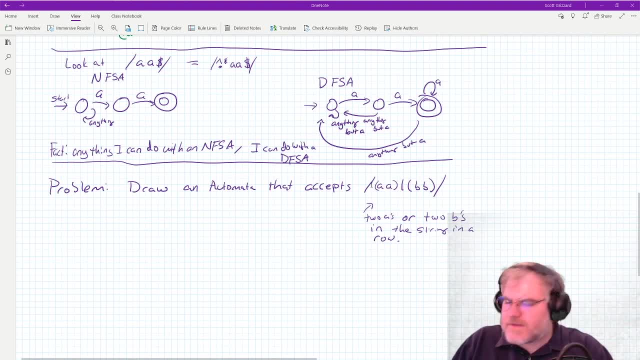 This thing: right here there's two A's or two B bits, Notice I've got no terminal and no, I've got no, you know, terminating point and no initial point. So that's the exact same thing as saying this: Okay, 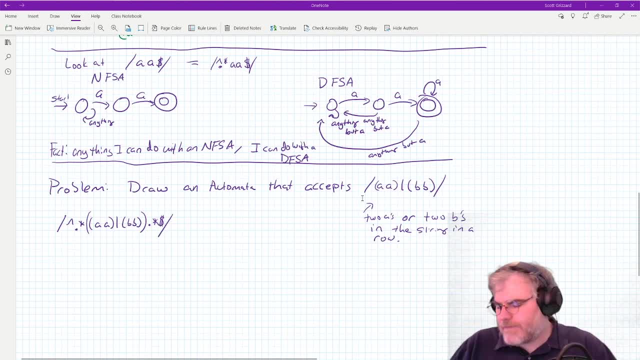 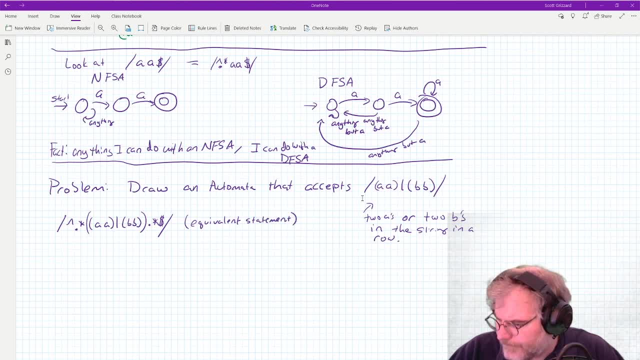 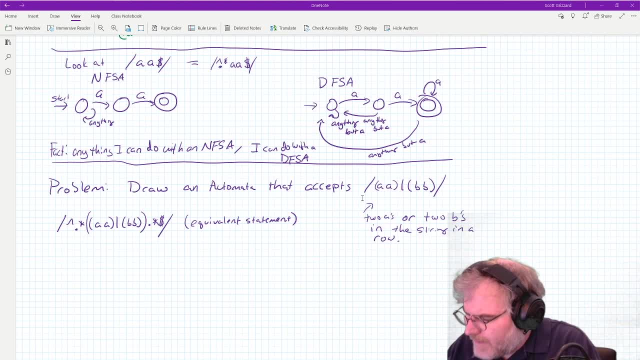 non-deterministic finite state automaton. I might have a concluding state here within anything. All right, All right, All right. now I'm going to have a B and a B, and then I'm gonna have a concluding state here, and then anything whenever they never have a day, and then I'm gonna have. 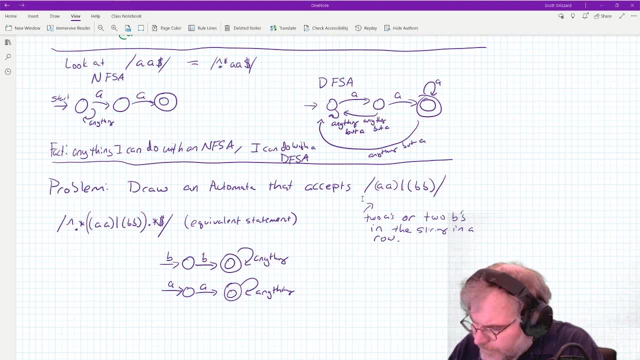 a start within anything. okay, how do we feel about that? one to five? well, this match my regular expression. now I can do something really clever. right here. I'm gonna get some bells or Mantell candles, and this episódio now does that right match my regular expression. this is one machine. 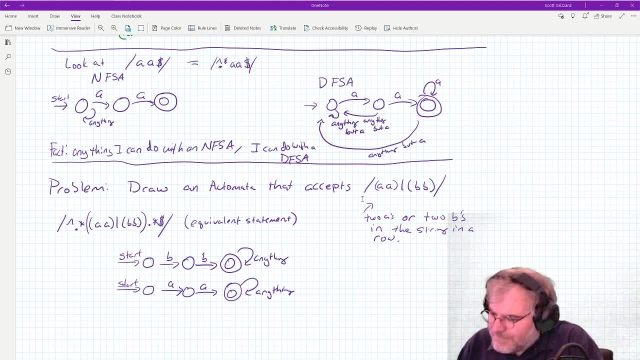 you, anything with two B's will match and anything with two A's will match, kind of slick, huh, okay, in other words, a non-deterministic, finite state of automata is a beautiful way to deal with. or statements: right, this is beautiful. right, it's got to match one of these two. 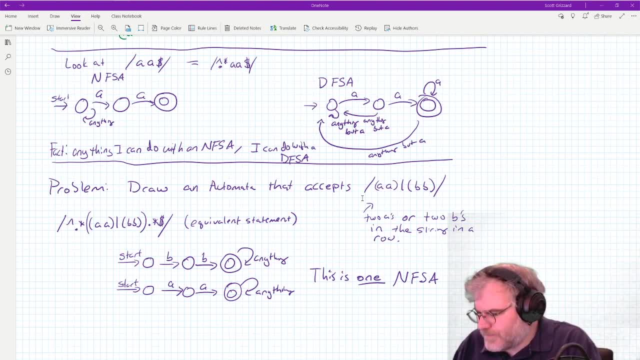 right. how do you feel about that one to five? what's more, going back to the question above that I can't mention, there's an algorithm for converting finite state, for converting regular expressions right to non-deterministic finite state automata. okay, well, so there's a question. 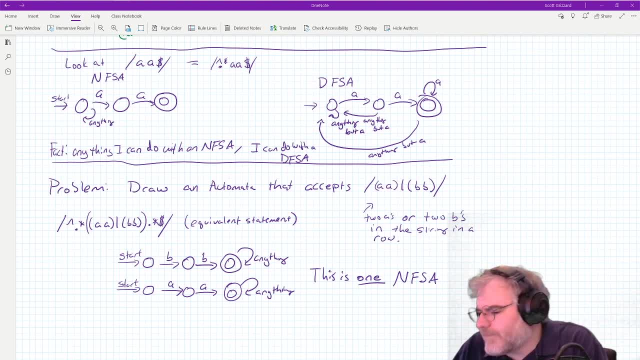 do I need a junk state in this problem? remember, junk states are optional to begin with. I'm just throwing them in there because- but they're usually for a non-deterministic automata. you don't write it in there. okay, you actually don't technically need to write it. 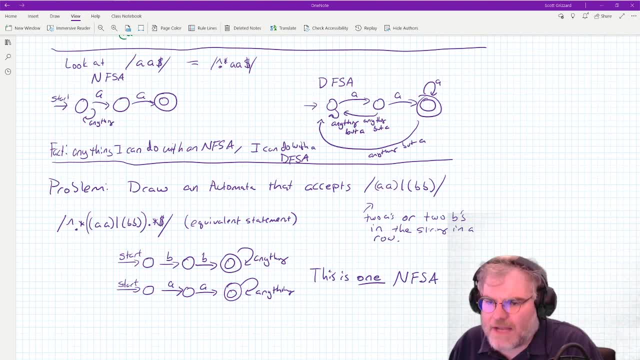 even for a deterministic finite state automata, because you just start throwing out bad stuff, because the junk always does basically the same thing. the only time I really care about a junk state is when I'm doing compliments, because when I'm doing compliments I want to accept junk. 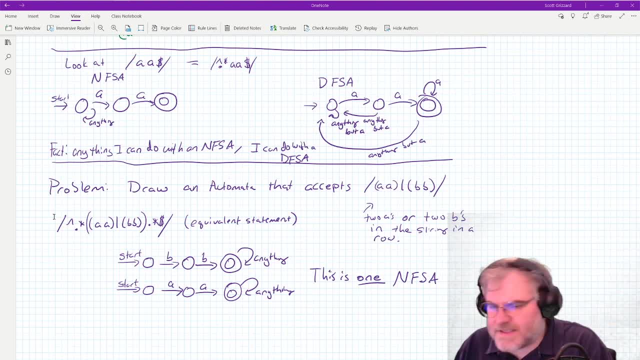 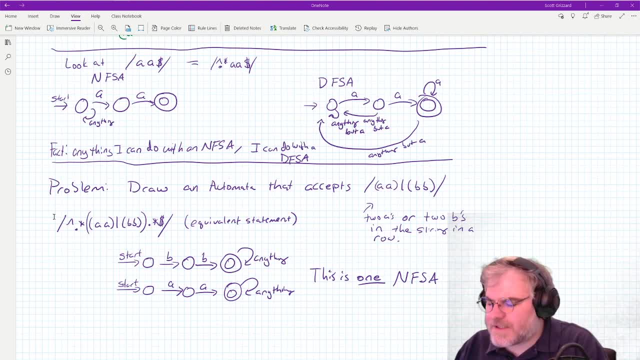 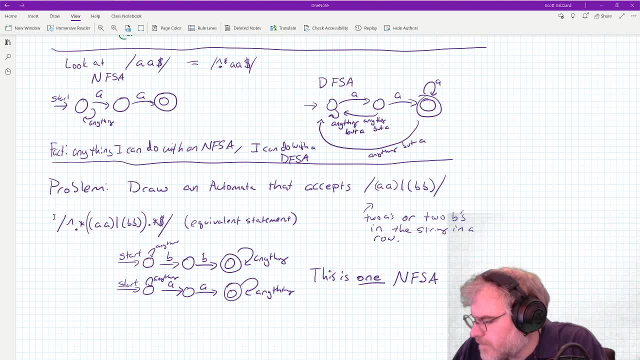 all right, I'm going to start with the junk state. um, now to answer that question, which I was doing before, there's an easy algorithm to convert regular expressions to non-deterministic finite state automata, and then there's an algorithm to convert non-deterministic state of finite state automata. 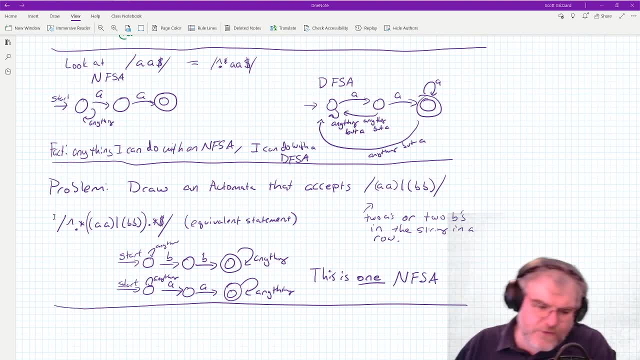 to um, to deterministic state of finite state. automata book is long and even more boring than the regular version. Klein's theorem. how part of Klein's theorem works? Klein, I guess, is his name. There's an algorithm To convert NFSA. there's an algorithm to convert RegEx to NFSA. 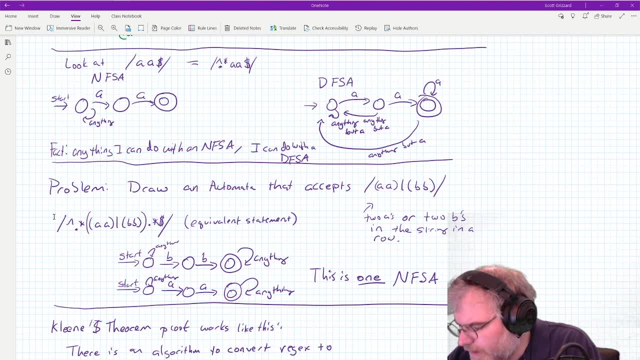 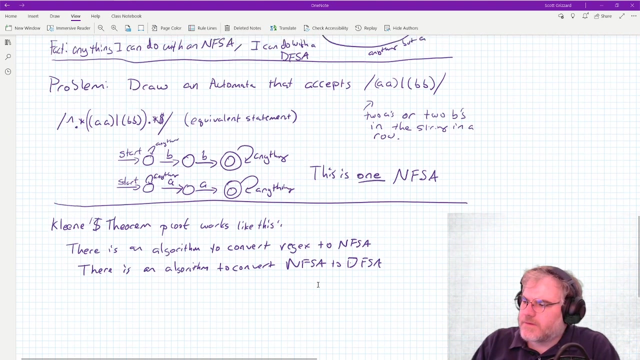 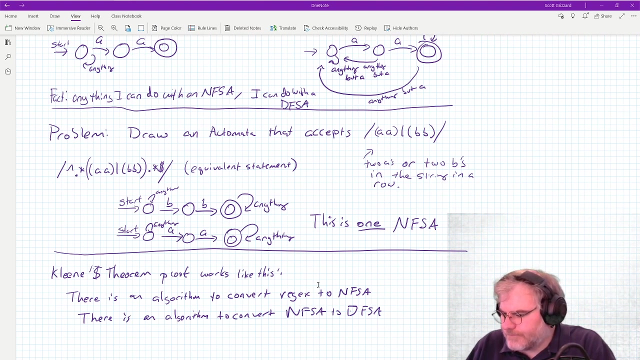 Okay, there is an algorithm to convert NFSA From FSA to DFSA. Okay, That's basically how it works. All right, are there any questions about this? Okay, Okay, So everyone feels comfortable with this idea that I could give them a non-deterministic finite state automata. 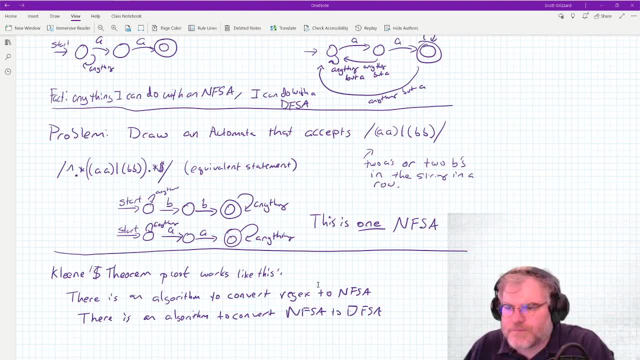 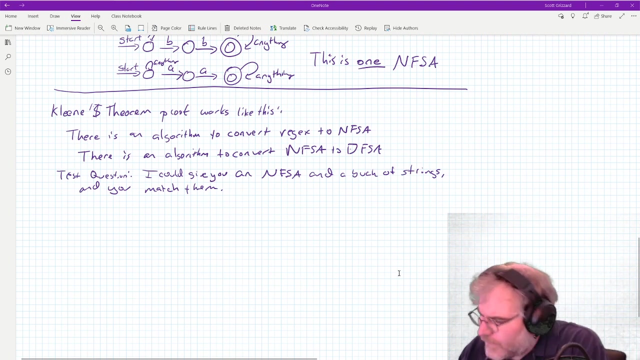 and a bunch of expressions and you tell me if they match. Okay. Okay, Thank you, okay. so that's a good test question. all right, let's talk about NP. there are these things called Turing machines, and you will see Turing machines again, okay. 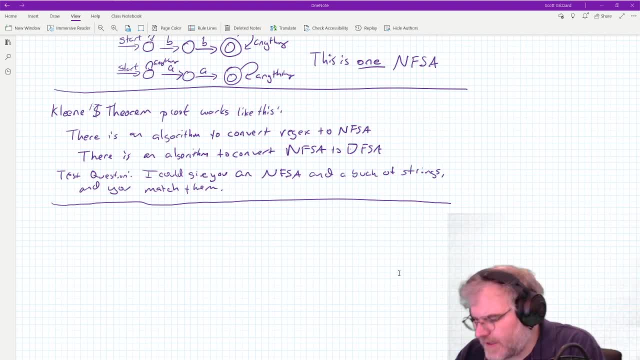 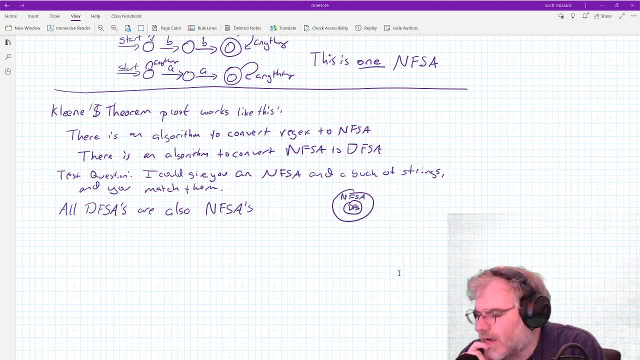 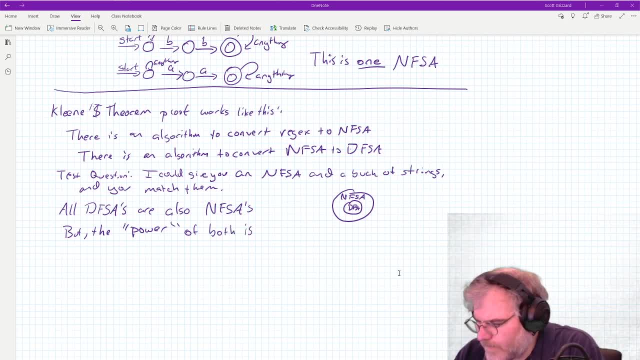 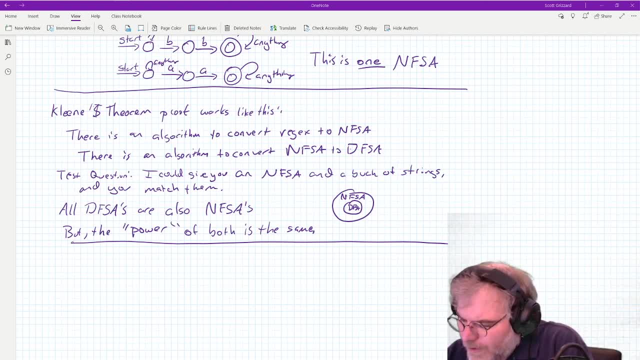 now, how much time do I have left? I have five minutes, I'm not gonna get through it. equals NP. now, how much time do I have left? I have five minutes, I'm not gonna get through it. equals NP, all right, so we call a problem. We call it a problem in P if it can be solved by a deterministic. 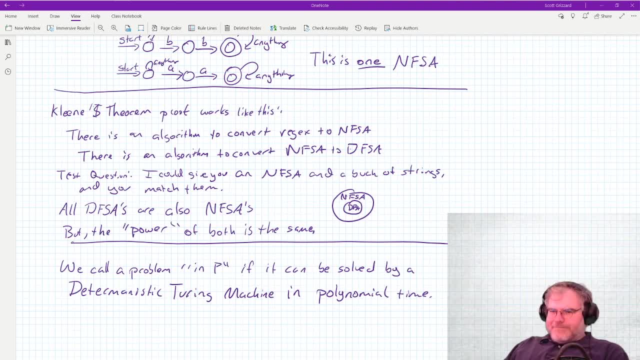 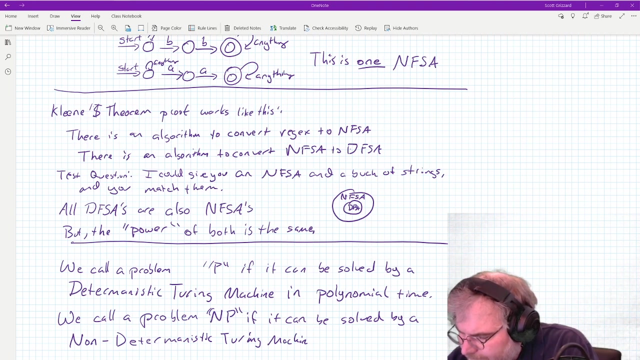 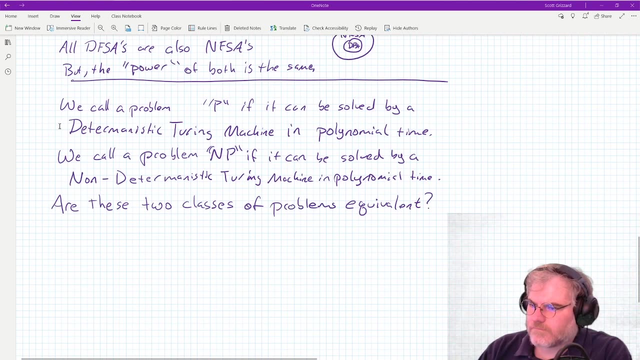 Turing machine in polynomial time. Okay, We call a problem or just P. We sometimes just say P If it can be solved By a non-deterministic Turing machine. Yes, this is polynomial time. That is the million dollar question. 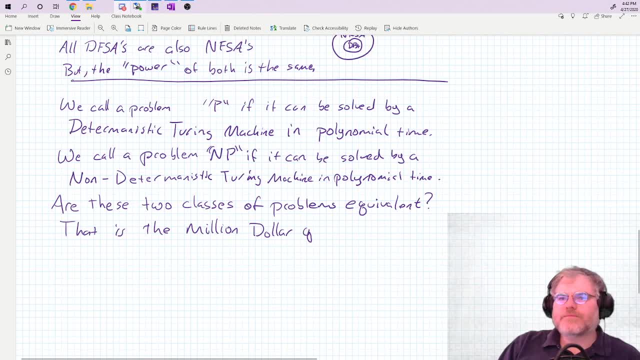 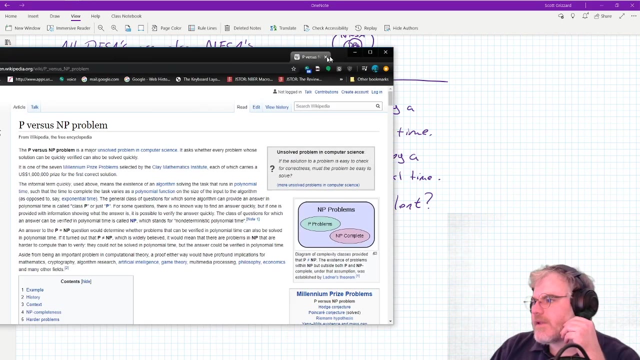 No, really, it's the million dollar question. All right, And that's where we'll stop on this thing. Okay, If you want to read about this, the Wikipedia article is actually pretty good. The question that you have to understand is: 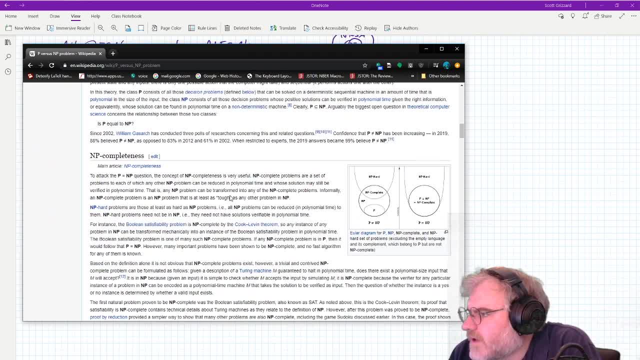 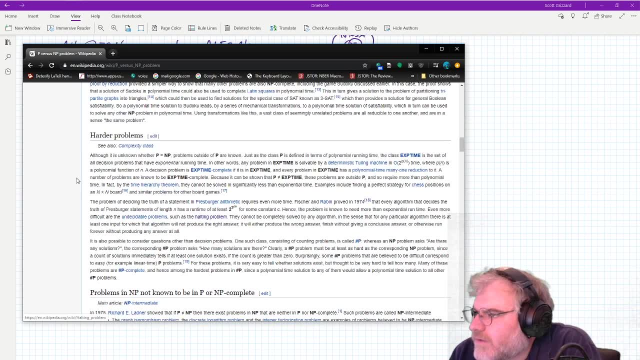 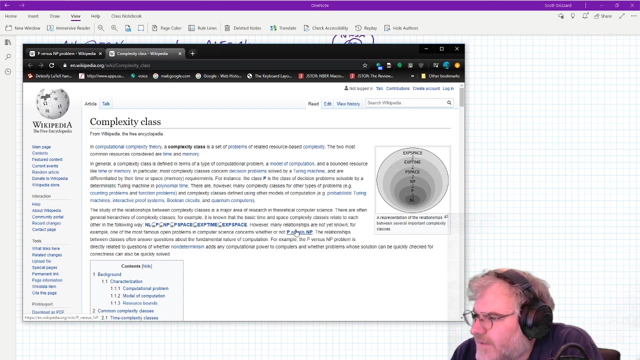 the thing you really need to understand is what is meant by a non-deterministic machine. Okay, So we have this hierarchy of complexity, classes, Okay, And we actually don't know where the, where, the, where the inclusions are. We know that this level at the bottom does not equal. 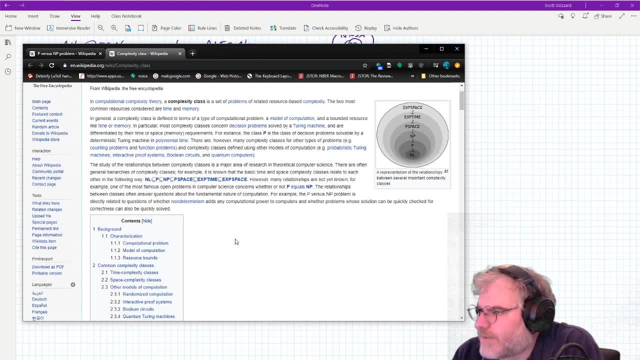 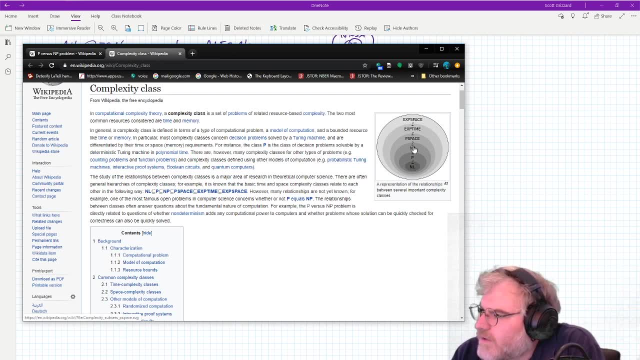 this level at the top. We have no idea which ones are not equal. We think that P is a strict subset of NP, but we don't know. We do have. and we also think that P is a strict subset of PSPACE, but we don't know. Alright, and that's the big. 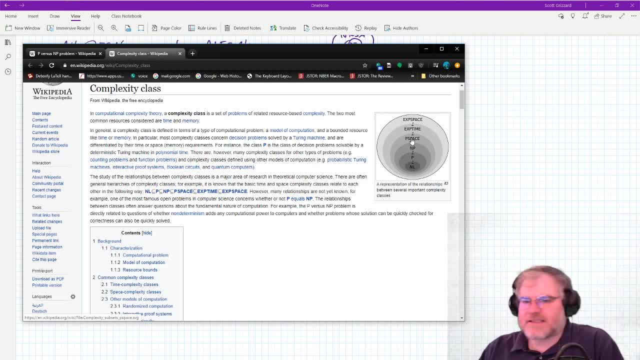 million-dollar question. We don't know. If you want to read about complexity classes, you can get obsessed with this stuff. Go ahead. it's kind of obsessive stuff. It's really weird that we don't have a proof for this, that we don't know. 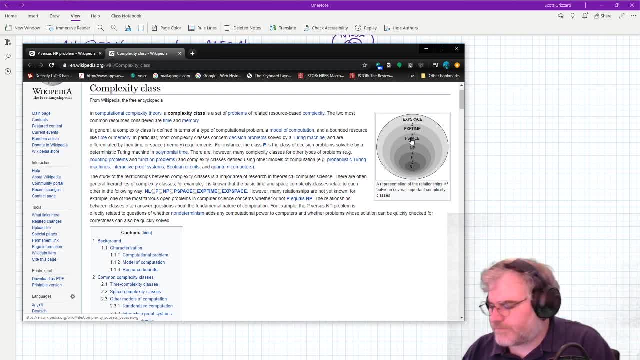 We do know that diagonalization, we do know that NP-space and polynomial space are equivalent. okay, So the amount of memory that each would have to have is. I mean, the amount of memory is not equal, but it's polynomial, so things tend. 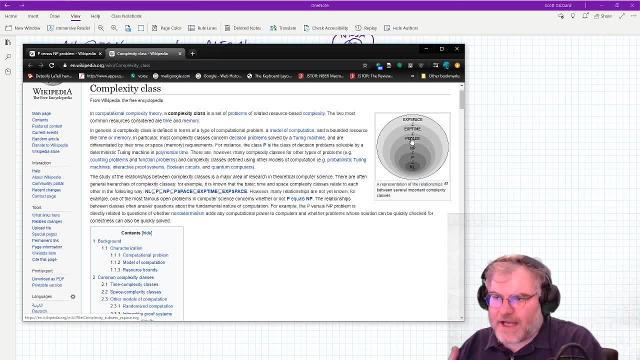 to grow like more and more Moore's law are exponential laws. okay, So we know that computers get more and more efficient exponentially, And so anything that you can solve in polynomial time is going to be solvable at some point in the future. 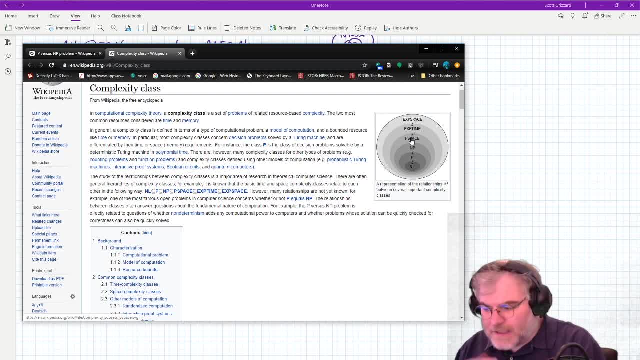 And we call these problems easy. Now those polynomials can be really, really big, But the idea is that computers get faster and faster, exponentially. Therefore at some point we'll be able to solve it, Whereas anything that's exponential time in origin. 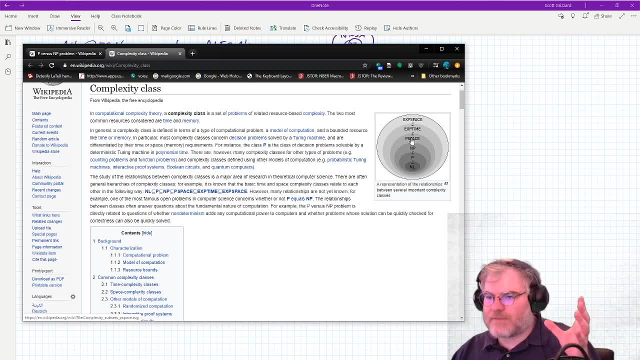 you can just keep adding more things to the problem, And it was. You can just add more time to the problem. Yeah, p space is equal to np space. Okay, are there any questions about that? Well, it's a place to leave it.